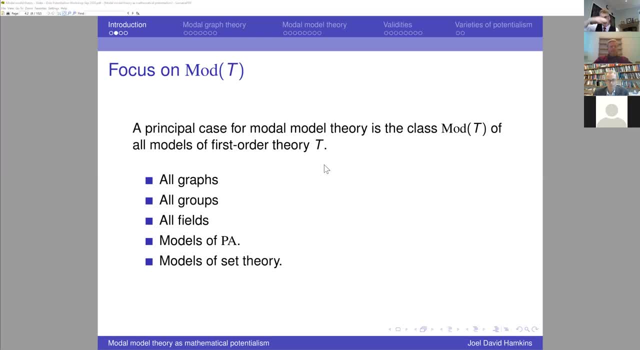 potentialism set theoretic potentialism in that paper. There's rank potentialism, There's topic potentialism, There's submodel potentialism, which is what I'm talking about here, There's foreseeing potentialism and so on. There's all different kinds of potentialism And in the case 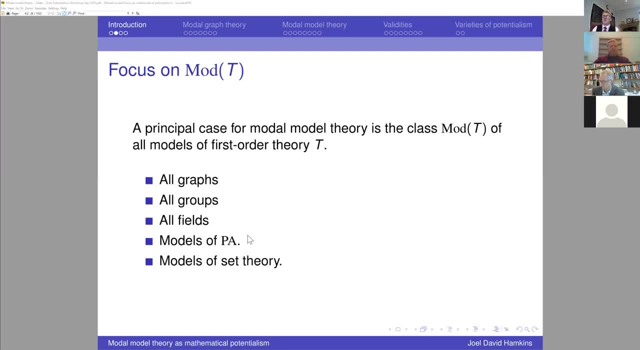 of arithmetic, for example. there's also different forms of extension. Maybe you want to look only at end extensions of models of arithmetic, or do you want cofinal extensions and so on. This has to do with the idea of whether or not, for example, in your arithmetic potentialism. 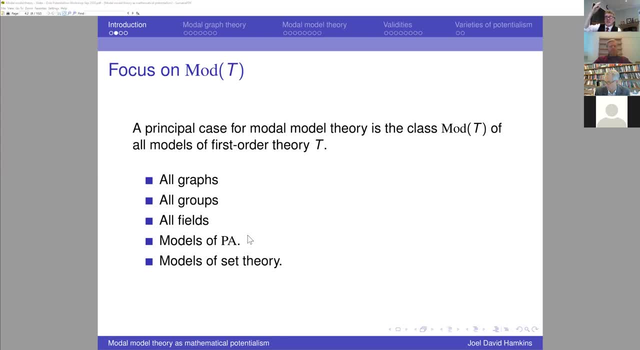 you allow that numbers come into actual existence And then, later on, smaller numbers might come into existence that weren't actual at the same time. For example, maybe it's reasonable to say that maybe a googolplex becomes actual before some of the small, some of the smaller numbers become actual In terms of comodrop complexity, for example. 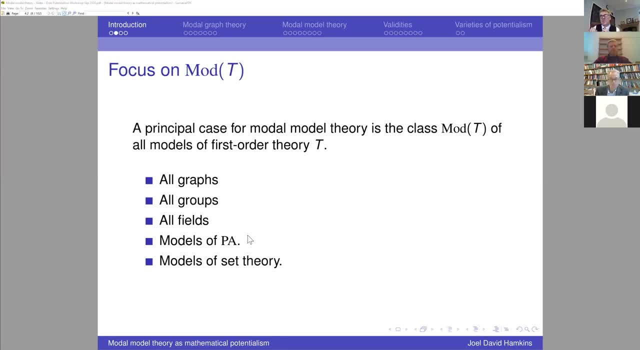 a googolplex is very low complexity, but some of the numbers that are actually smaller have much higher comodrop complexity, And so this is connected with that. Okay, of course, we can illustrate now the modal vocabulary in these mathematical contexts. So every graph thinks: 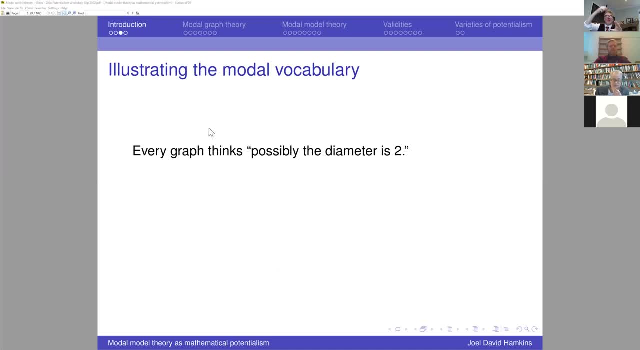 possibly the diameter is two because if I have any graph I can add another node and connect it up to the previous nodes in such a way that now in the larger graph the diameter is two, Or every group is possibly necessarily non-abelian, because every group is a subgroup of a non-abelian group. 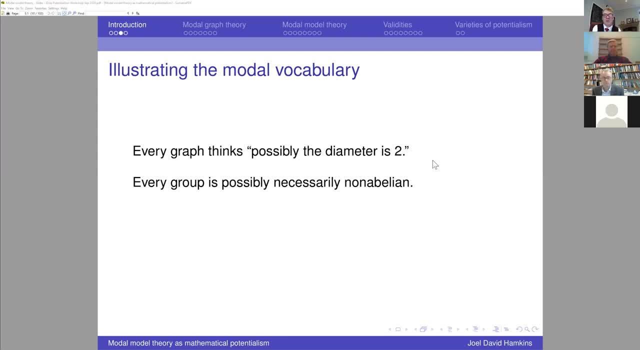 and then forever on. in any larger group it will still be non-abelian. Or every field thinks possibly every element has a square root, because you can take the algebraic closure of the field and that's a field that thinks everybody has a square root. But this is necessarily not necessary. 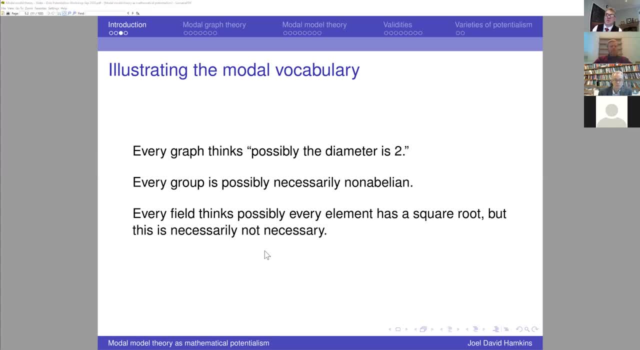 because every field also has a transcendental extension in which it's not true that everybody has a square root. Okay, I want to particularly distinguish several different languages. Of course there's the base language of the structure, So maybe L is the language of set theory. 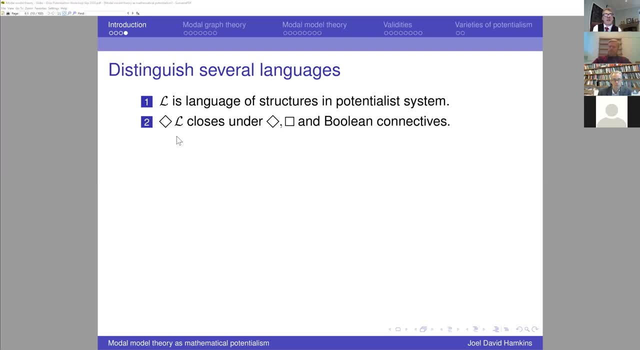 or the language of arithmetic, or the language of graph theory. There's this intermediate modal language which we call diamond L, which is where you close L under the modal operators and Boolean connectives, But you don't close it under quantifiers. so there's no. 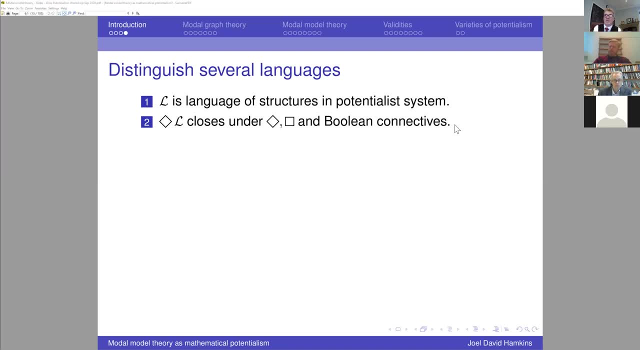 modal operators under the scope of a quantifier in this language, Then the full modal language closes under everything. And then also maybe you want to add an actuality operator, which I'll talk about briefly. That's an extension of this full modal language. And then there's the propositional. 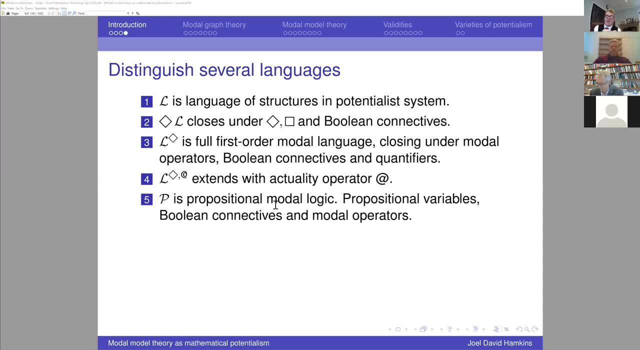 modal logic. This is the language that has propositional variables and then Boolean connectives and modal operators, only no quantifiers or variables. So, for example, this diamond L language is exactly what you get from the propositional assertions by substituting in L sentences. That's what it would take for the modal operators to never be under the scope. 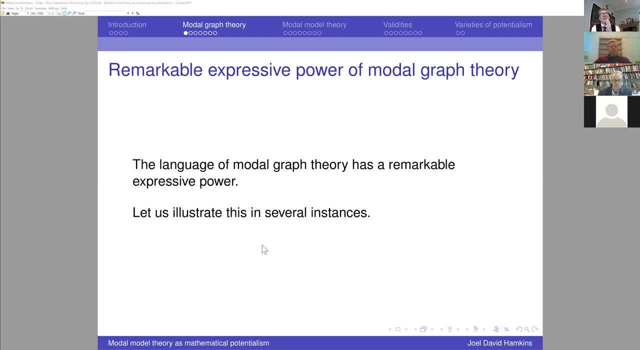 of a quantifier. Okay, let's look at modal graph theory. So this is sort of potentialist graph theory and I want to explore a little bit the remarkable expressive power of modal graph theory. So, for example, two colorability of a graph. 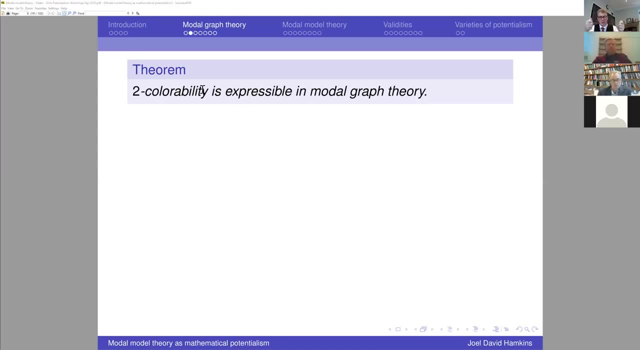 is expressible. So a graph is two colorable, if you can color the vertices, say red and blue, so that nodes that are connected by an edge don't have the same color. And this is expressible because you can say possibly. so here's the graph G. 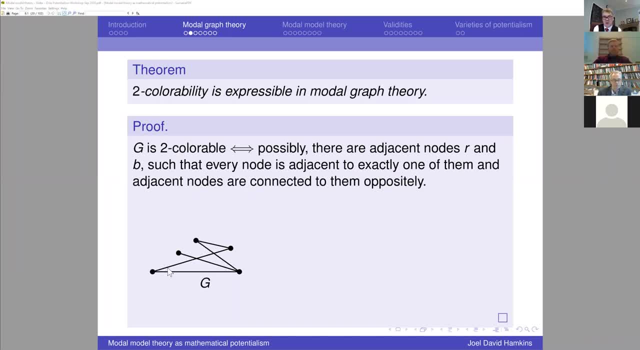 this graph is two colorable, because I could make these ones all red and I could make these two over here blue and that would be a coloring of that graph. But I can express this modally by saying: possibly there are adjacent nodes R and B, such that every node is adjacent to exactly one of them. 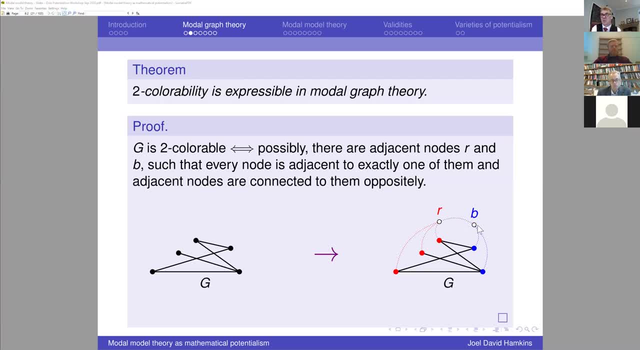 and adjacent nodes are connected oppositely. So here's R and B. I think of everybody that's connected to R as being colored red and everyone that's connected to B as colored blue, And so if there is a coloring I can add that to the graph. But I can express this modally by saying: possibly. 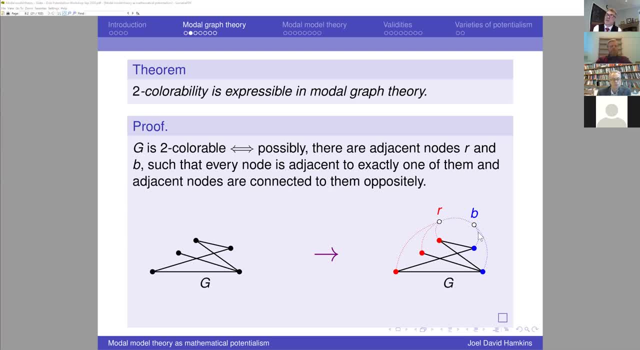 I can add nodes like that, and if I can add nodes like that then there must be a coloring, because I can get a color from that situation. Two coloring is not expressible in the language of graph theory, So this shows that the modal language is strictly stronger. 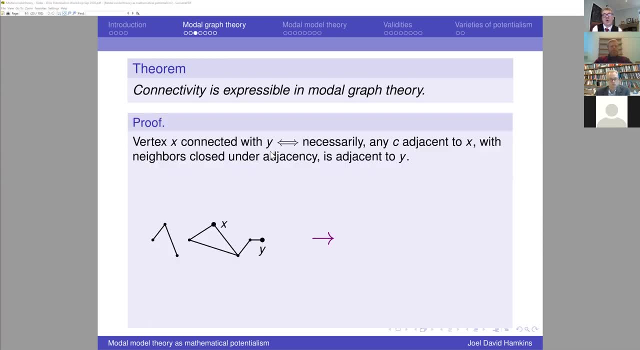 But also connectivity is expressible. For example, X is connected to Y in a graph just means that there's a path from X to Y, a finite path along the edges, And you can express this as kind of like induction. So necessarily any vertex C that's adjacent to X and whose neighbors. 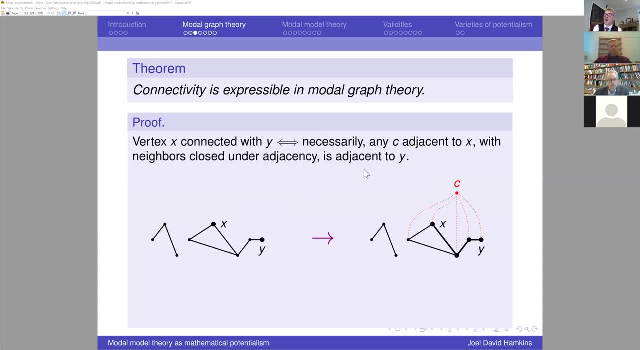 are closed under adjacency will also be adjacent to Y. So if they are connected, that's certainly going to be true, and if they're not connected, I could add a vertex that was connected only to the component of X and it would be closed under adjacency. 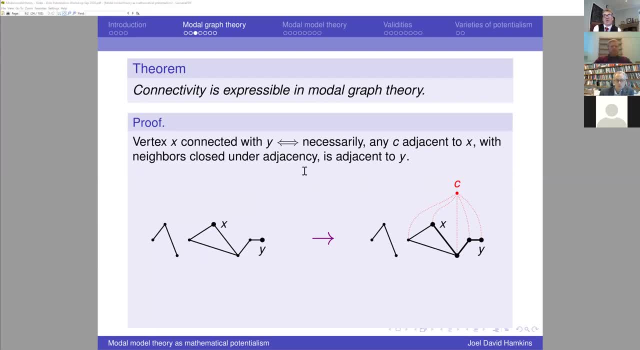 but it wouldn't be connected to Y and so therefore this is equivalent to being connected. Okay, Connectivity also is not expressible in the language of graph theory, So this is the formal expression in the modal language. So finiteness is expressible. 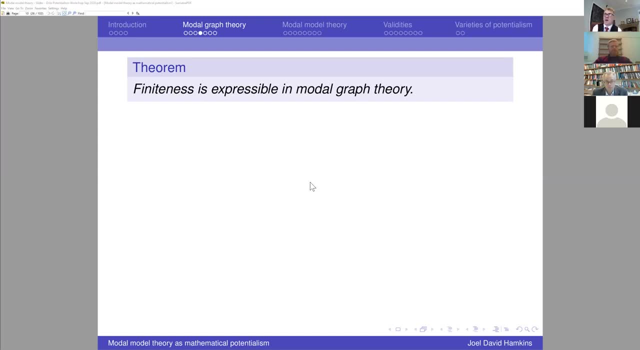 So again, of course, finiteness in any first order of theory, with infinite models, is not expressible. So this again shows that modal language is exceeding the regular one. So I claim a graph is finite, just in case possibly there's a point whose neighbors 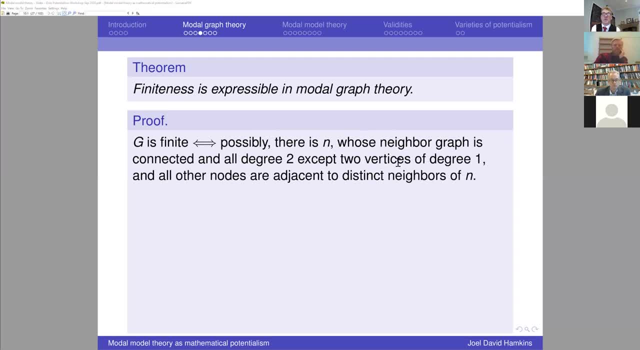 are connected and all have degree 2 except for two vertices of degree 1, and all the other nodes are adjacent. So here's the original graph. I'm saying possibly there's a node n whose neighbors are connected and have all degree 2 except for a starting node and an ending node in that neighbor set. 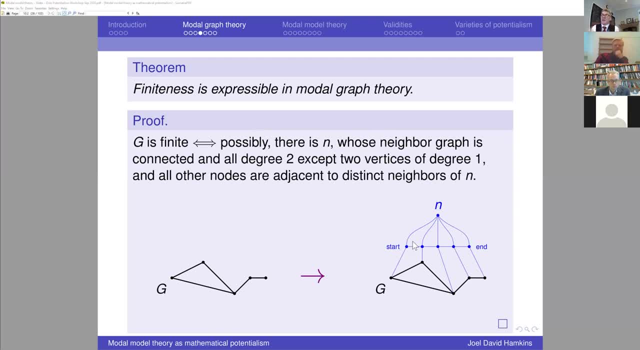 So that would have to be a finite chain from the start to the end. And then I'm saying such that all the other nodes are connected, All the other nodes are adjacent, adjacent to some of those neighbors of n. So this is exactly expressing the finiteness of 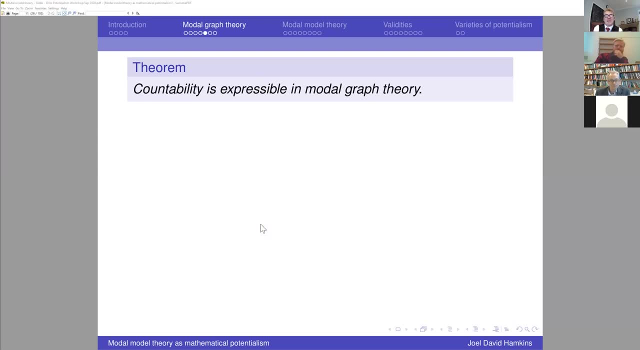 the original graph. You can also express countability in a similar way, So a graph is countable. just in case possibly there's a node omega whose neighbors are connected and all have degree two, except for one node which has degree one and everybody else is adjacent to. 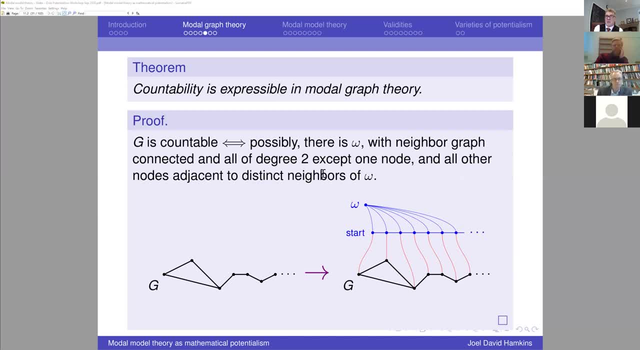 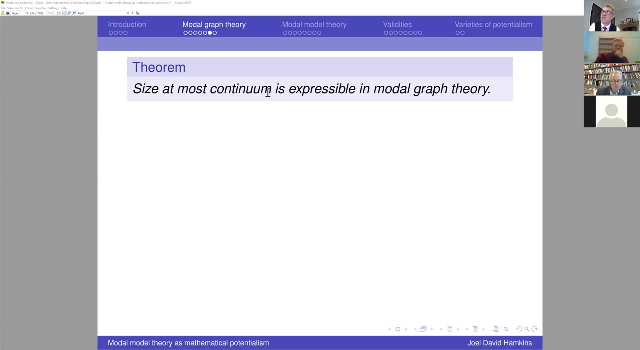 neighbors over mandarin. So this omega chain has to be a countable sequence and if everybody is adjacent to distinct members, then the original graph must have been countable and that's economic. Well, we can push this further. So having size continuum, at most continuum is expressible. 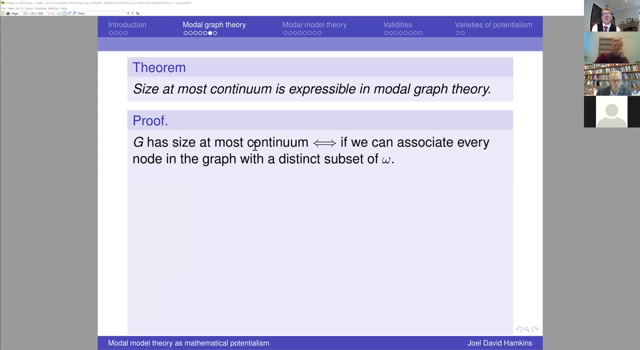 in modal graph theory. So a graph has size, at most continuum. just in case, you can associate to every node in the graph a distinct subset of omega, And so we can say: possibly there's a node omega whose neighbors are connected and all have degree two, except for one node which has degree one, I mean in the neighbor set, so that any other two 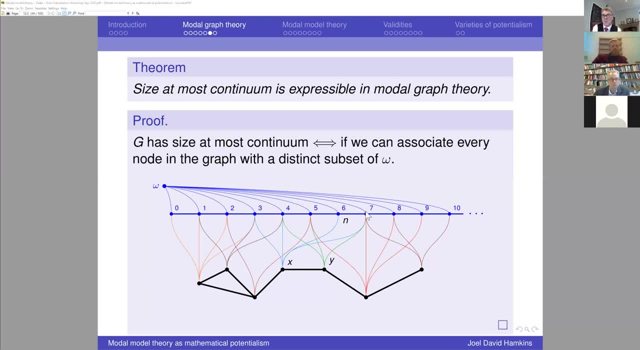 nodes like x and y are connected to distinct subsets of neighbors of omega, So x and y differ on their connectivity to this node n, and so that means that we've associated to every node a subset of that countable set, and so the graph would have to have size at most continuum. Okay, one can push. 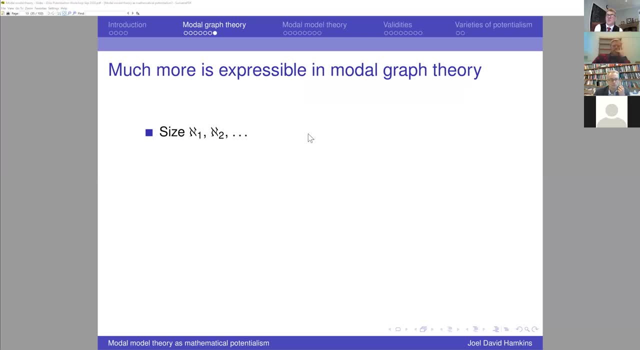 this very, very far. we can express having size of one or two and so on, all of omega vaccine. We can express having the size of the least that fixed point or the least hyperfixed point, and so on, much, much more. So modal graph theory is incredibly expressive. 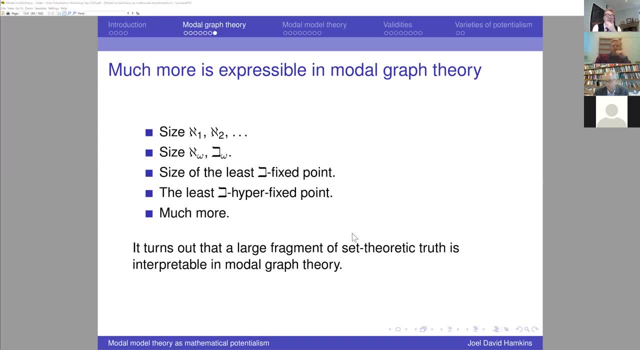 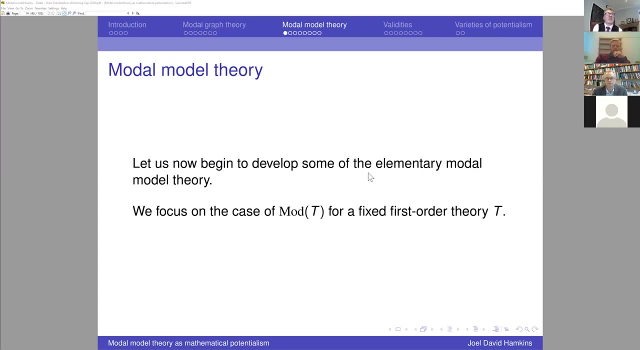 in terms of these set theoretic uh features, and a large fragment of separate truth is in fact interpretable In modal graph theory. you can interpret much of set theory into a assertions about graphs in the model language of graph theory. Okay, let's now go to the sort of more general case of modT, the set of models of the first. 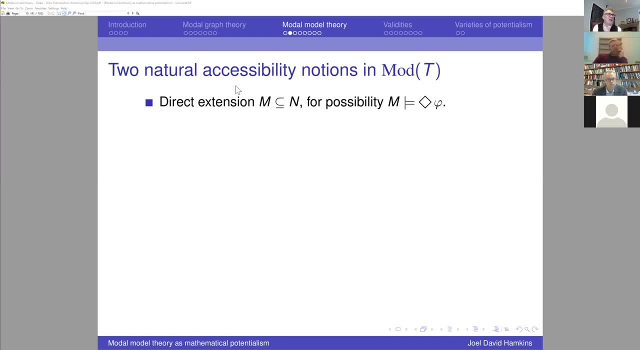 order theory T. So I want to emphasize that there's two natural accessibility notions in modT. On the one hand there's direct extension, which I think is what many potentialists are usually thinking about. So something is possible if there's some extension. 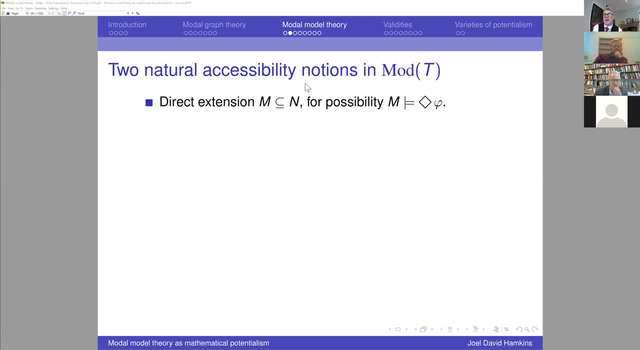 So M is a substructure of N, and N satisfies T, And this is very natural from a potentialist point of view. You think of the individuals as coming into actual existence, and then those individuals persist as the very same individual. But there's a problem with direct extension in that it has very poor algebraic properties. 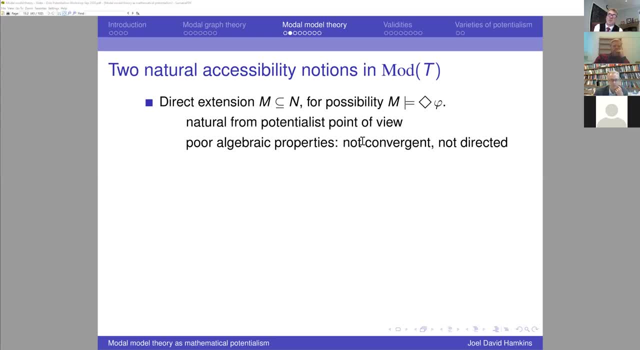 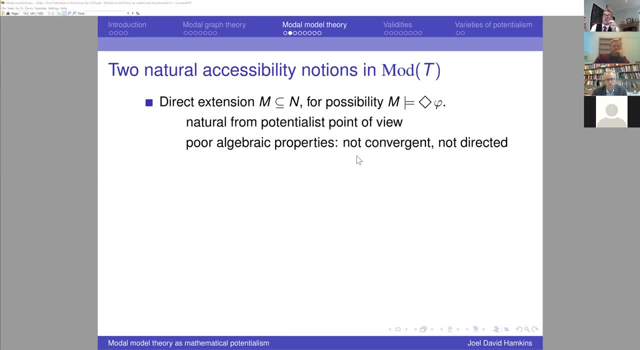 or you could have used that same object, that same individual, in a different extension but in an incompatible way, And then there would be no way of bringing those two direct extensions together. And so if you want to argue, say for S4.2 because of directiveness, then if you're using 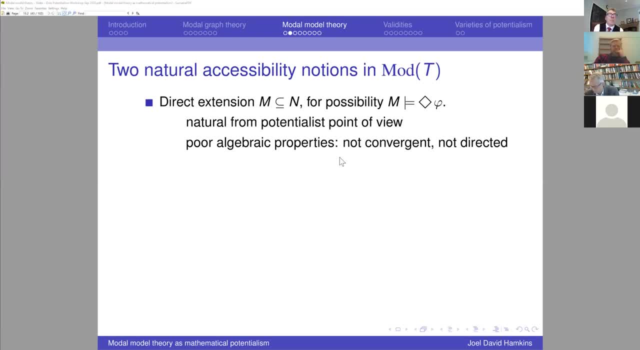 direct extension. you're not going to have it, And so there's another way of talking about it, And that is embedded extension. So an embedded extension is where M is isomorphic to a substructure of M. So we have an isomorphism, an embedding of M into M. 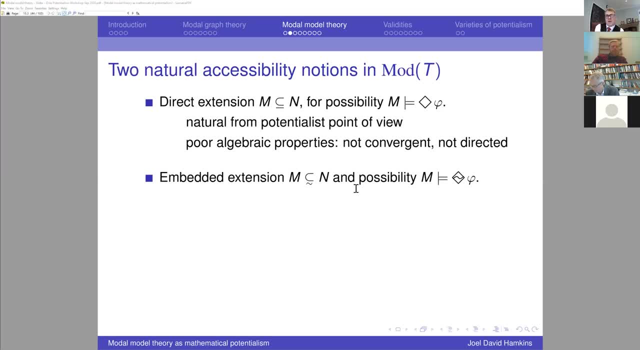 And now this is embedding possibility, And this is very natural from a mathematical point of view. Mathematicians often like to just look at things up to isomorphism and so on, so they want to think about embedding the structure instead of directly extending the structure. 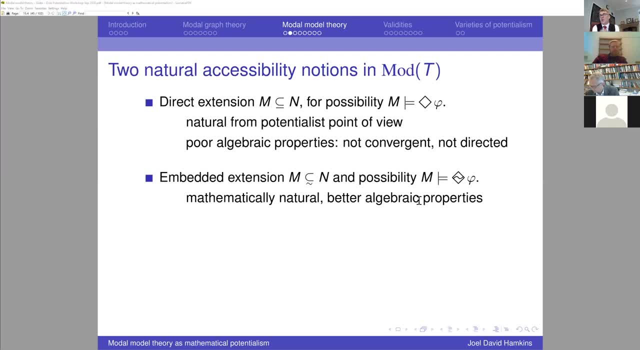 And also it has much better algebraic properties. For example, in many natural cases it does have convergence, it does have amalgamation, it does it is directed, and so on. And then the observation is that, fortunately, the two modalities are identical. 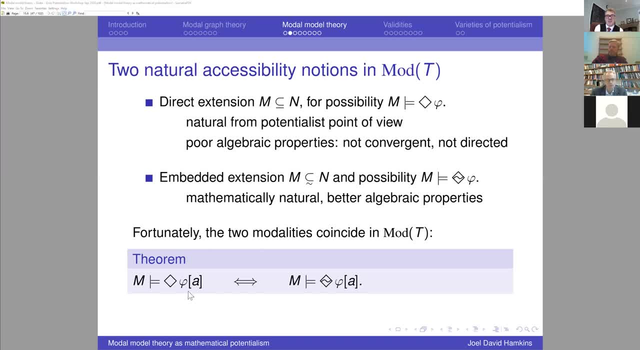 And so so something is possible with direct extension, if and only if it's possible with embedding extension, And so this tells us: well, we don't actually need to worry if we're just talking about modal assertions, We don't need to worry about the difference. 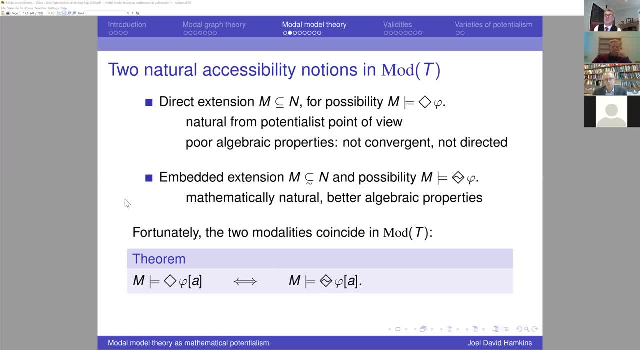 Right, There's a difference between direct extension and embedded extension, And the point of this is that now we can think about direct extension as the main extension, but we can use the algebraic properties of the embedded extension, which is directly an amalgamation, and so on, in order to make conclusions about the nature of the modal. 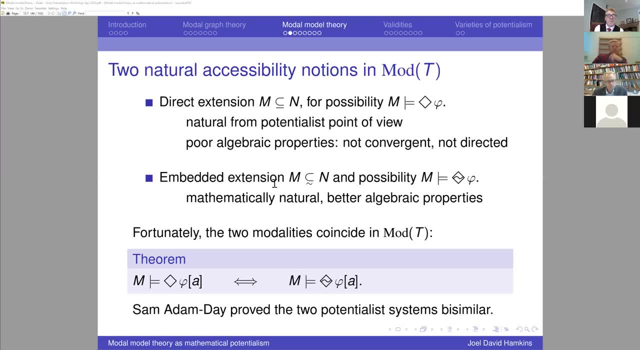 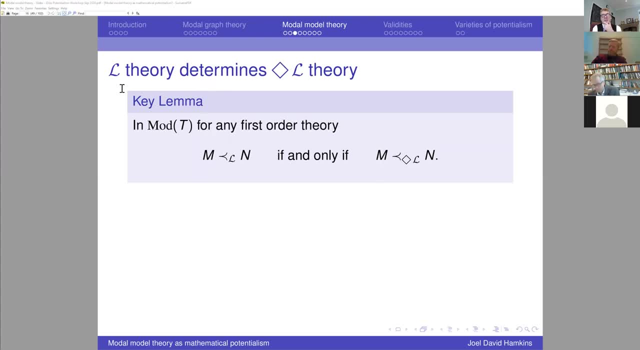 features of the direct extension. Okay, so now. one of the first lemmas we proved about modal model theory is that the, the, the L-theory, determines the diamond L-theory. This is the intermediate modal theory. So if you, if you have an elementary substructure in the, in the original language, then that 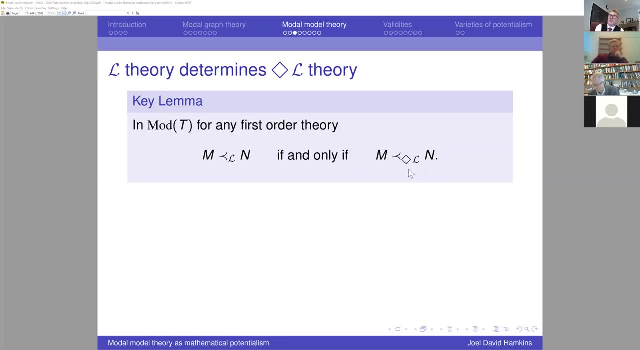 is if, and only if, it's elementary in the diamond L-language. So there's a sense in which the diamond L-theory, the modal theory in this fragment of the modal logic is completely determined by the L-theory. It's not true in the full modal language, but it is true for the intermediate modal. 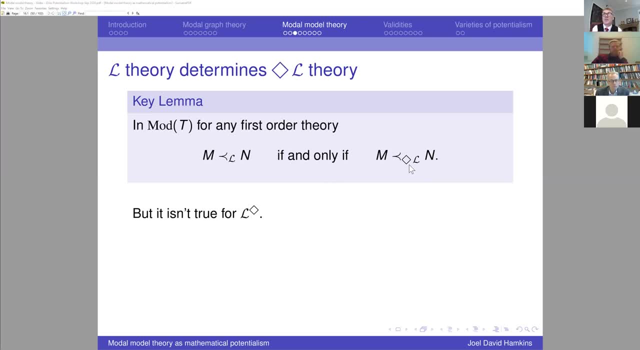 language, And that's one of the reasons to pay attention to this intermediate modal fragment. So it's also true for elementary equivalence. So if M and N have the same theory in the original language, then they have the same theory in the diamond L-language as well. 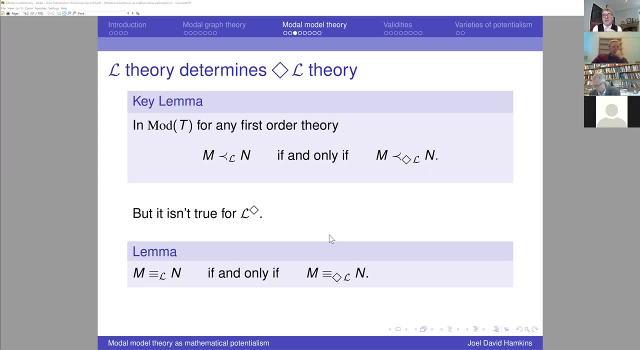 And you can use this to show, for example, that, um, countability is not expressible in the diamond L-language of graph theory. Okay, You can have a countable graph and an uncountable graph, having the same theory, uh, like by. 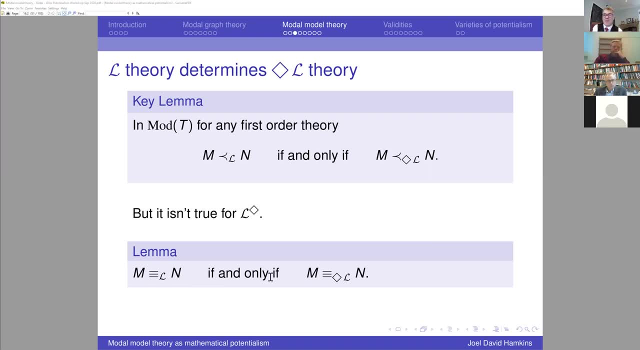 Leuvenheim-Scholem. That's true, Uh, but then therefore they would have to also have the same diamond L-theory, And so diamond L is not capable of expressing countability for that reason. So this is not true in the full modal language, because the full modal language was capable. 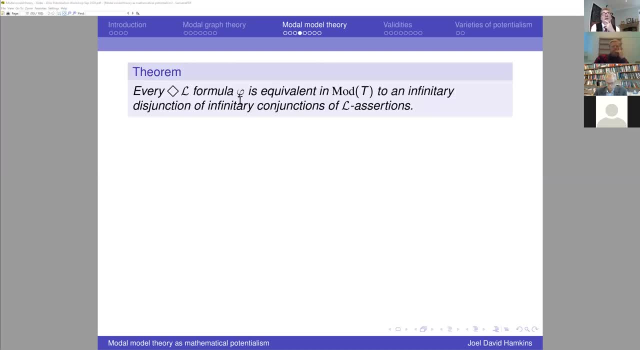 of expressing countability. Okay, So maybe that theorem suggests that because the diamond L-theory is equivalent to the um countability, I mean, as determined by the L-theory, you might think. well, that must be because the 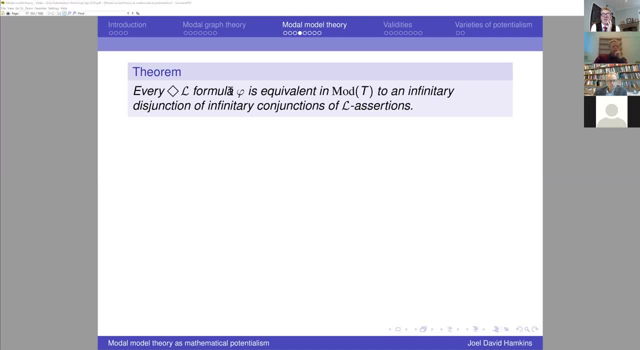 diamond L-theory is: uh, every diamond L-assertion is maybe expressible in the original language, but that's not true. um, because two colorability is diamond L-expressible, but it's not expressible in the language of graph theory. 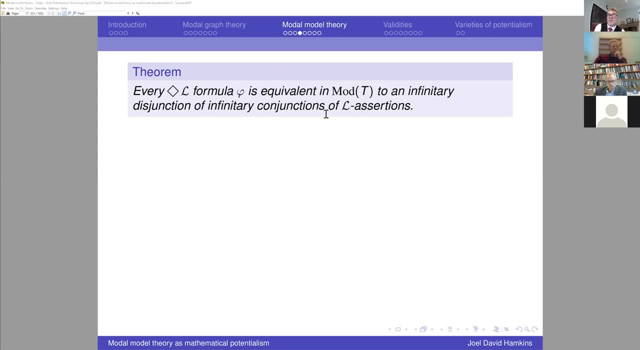 But meanwhile every diamond L-formula is equivalent to an infinitary L-assertion. And that's just because Whether or not a model satisfies a formula phi is determined by its L-theory, And so phi is equivalent to asserting of one of the theories of a model in which phi is. 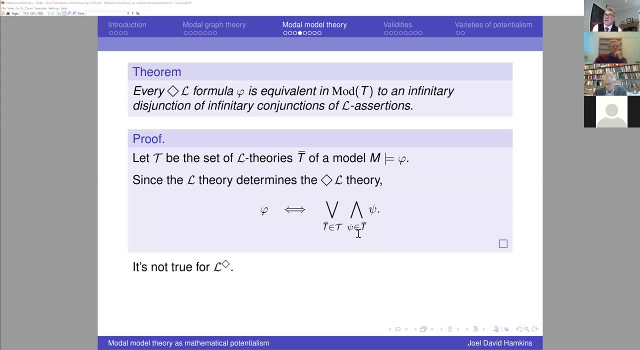 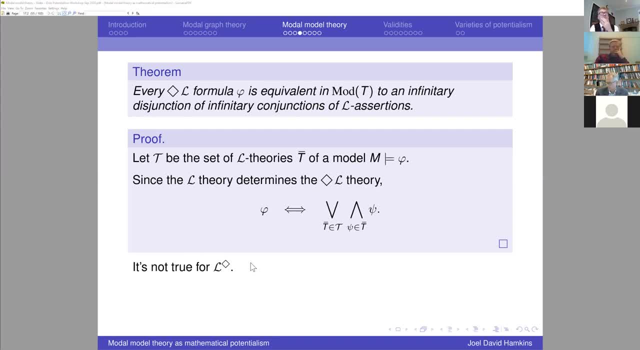 for those kind of accountability reasons that I just discussed. Okay, This equivalence, though, because this is a continuum size disjunction, this is a countable conjunction, So it's very natural to ask: well, is every diamond L-assertion equivalent to an assertion? 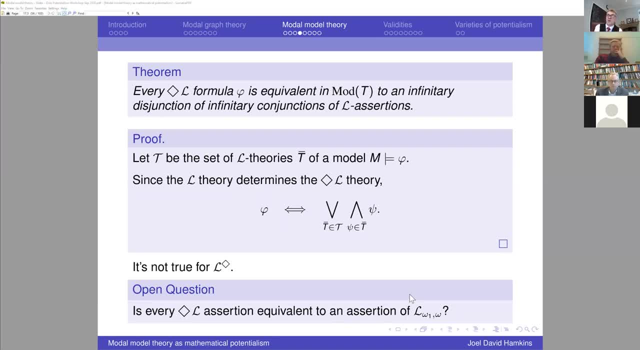 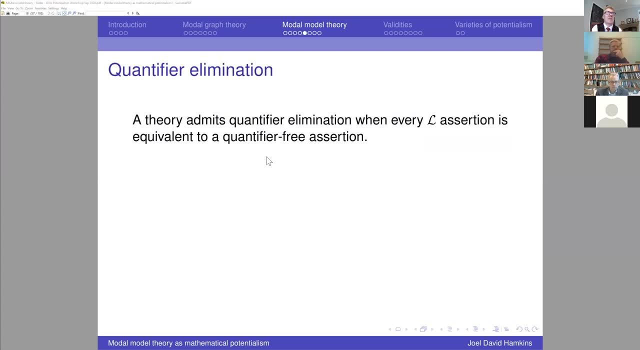 of L, omega, one omega, where you have only countable conjunctions and countable disjunctions And we don't know the answer to that. It's open. So there's some special cases. model for yourself And look at, For example, quantifier elimination. uh, a theory admits quantifier elimination when 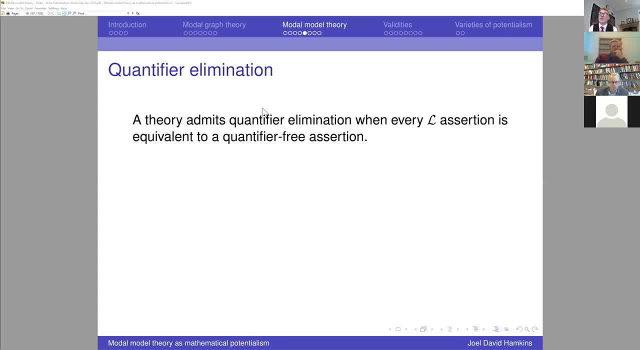 every L-assertion is equivalent to a quantifier free assertion. So this is true in very important, uh mathematical theories like endless dense linear orders or algebraically closed fields and so on, as many natural theories that admit quantifier elimination. And in those cases, uh, then we've proven that also you have modality elimination and 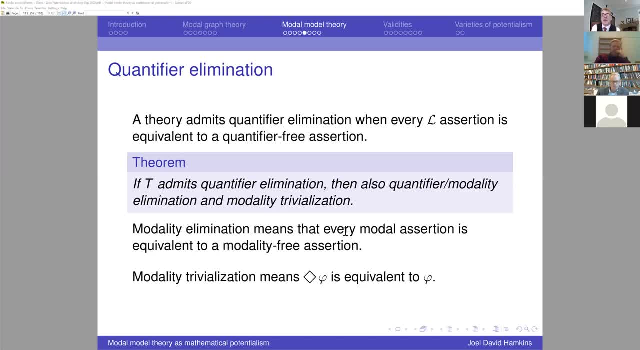 modality trivialization. So modality elimination, It means that every modal assertion should be equivalent to a modality free assertion. and modality trivialization means that, specifically, you can just delete the modalities and its equivalent so that the modalities are trivial. 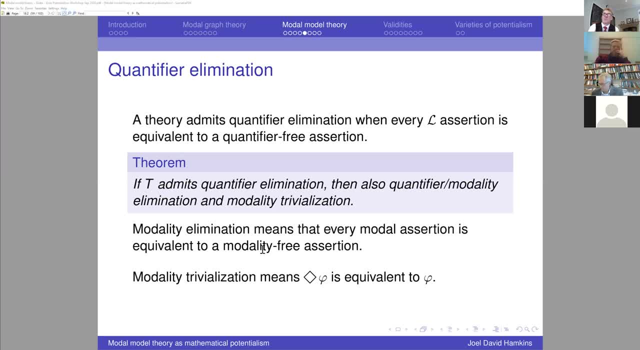 So we. so if the theory has quantifier elimination, then you shouldn't really be talking about the potentialist version, because the modalities become trivial. We can prove that modality elimination and modality trivialization are not equivalent. There's a 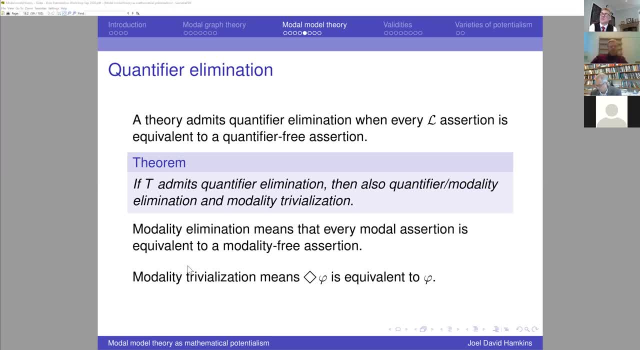 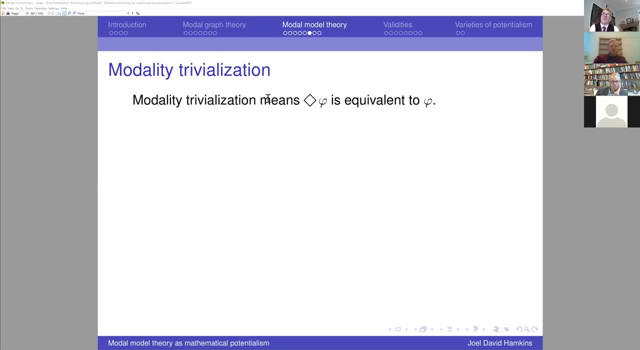 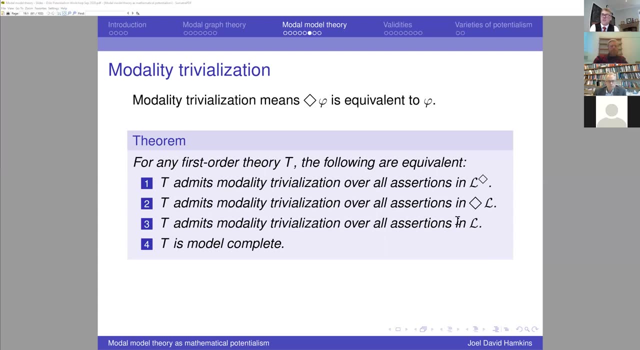 There's a theory that has elimination but not trivialization. So here's another, uh, necessary and sufficient condition for trivialization. So mainly, uh, the theory admits modality trivialization, and it doesn't matter whether you're looking at assertions over L or over diamond L or the full modal language. 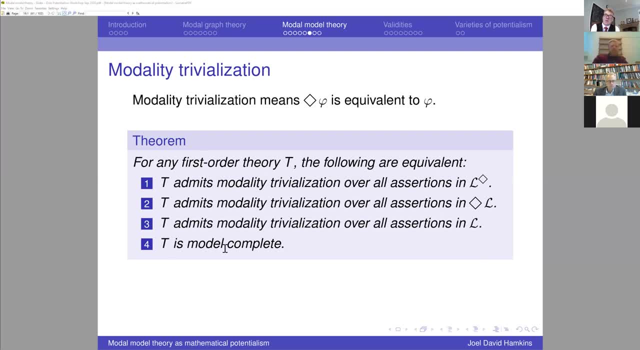 If you have modality trivialization in any of those, that's equivalent to the theory being what's called model complete. Model complete means that That substructures are automatically elementary substructures, So this is equivalent to the theory proving that every formula is equivalent to a universal. 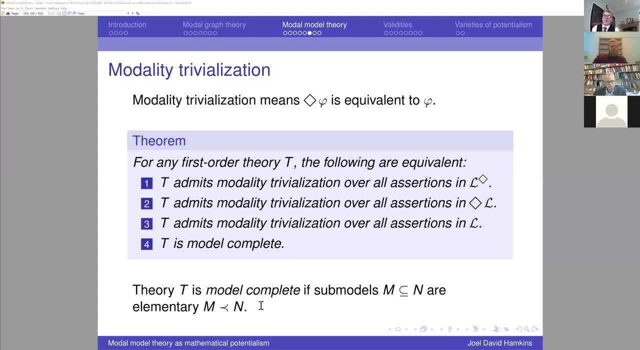 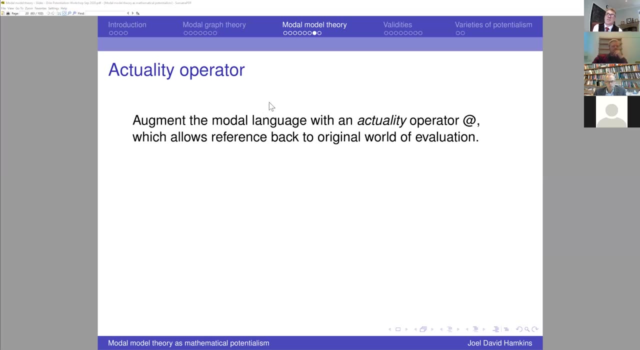 formula. So it's a weakening of quantifier. You can eliminate almost all the quantifiers, but you're going to have one universal quantifier. Well, it's natural to consider um, the actuality operator, and this is actually related to. 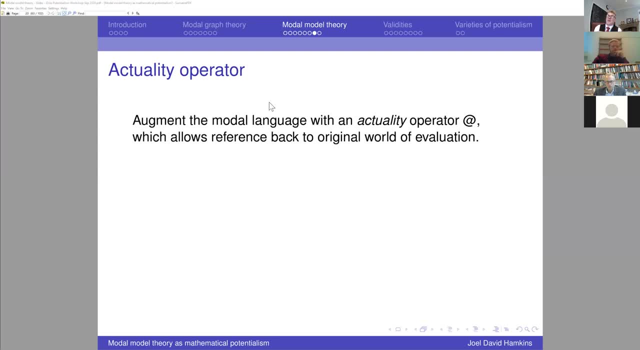 James, That question that he asked in the break, asking about where you are in the stages and so on, Actuality allows you, in effect, to refer back to the original worlds of of evaluation. So in the ordinary modal language, you are not able to say that it's possible that something. 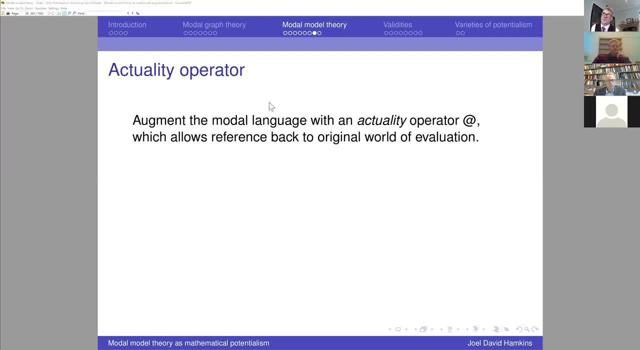 has a certain feature with respect to all of the objects that used to exist in the previous universe. You don't have any way of talking about the previous universe, and that's what the actuality operator allows you to do. So, for example, this statement here asserts that possibly there's a node adjacent to all. 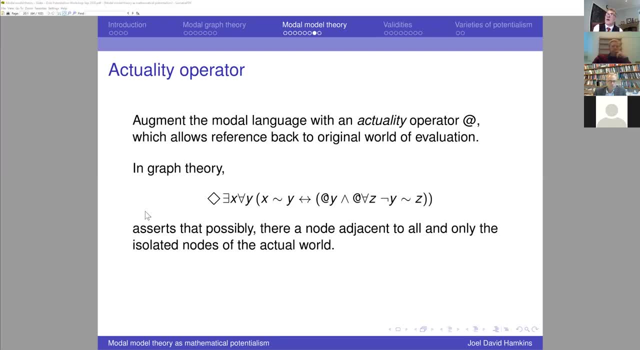 and only the isolated nodes of the actual world. I mean the nodes that are that are isolated in the world in which we're asserting this statement, not the world in which the the statement that's asserted to be possible is true. Okay, 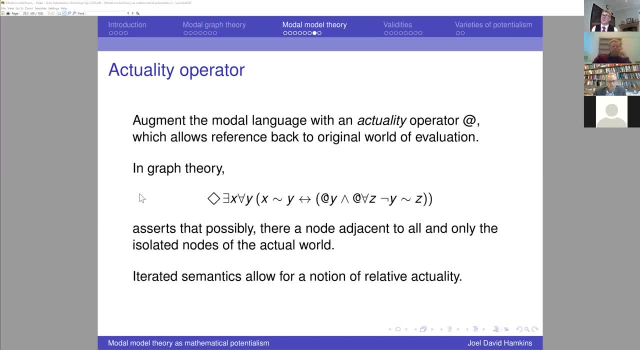 And then there's, of course, fancier versions with iterated semantics where if you say something is, say, necessarily possibly necessary, then you've got a whole sequence of worlds and you want to, You'll have actuality sub one and sub two, and so on you'll be able to refer back to. 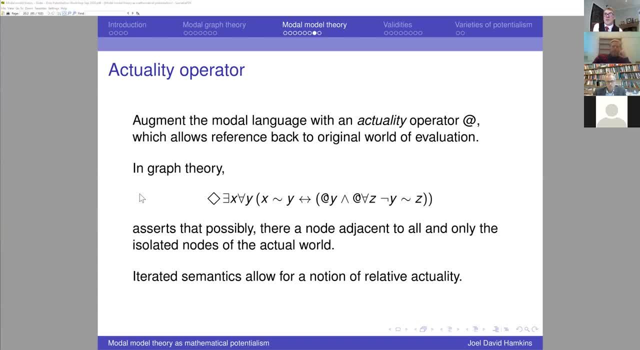 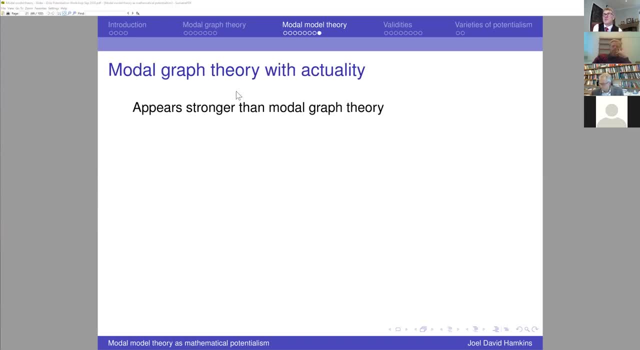 the worlds that arose during the semantical decomposition of the modal statement. So modal graph theory, with actuality, appears to be stronger than modal graph theory, although we can't prove that. So with modal graph theory with actuality, we can express: say that two nodes have an 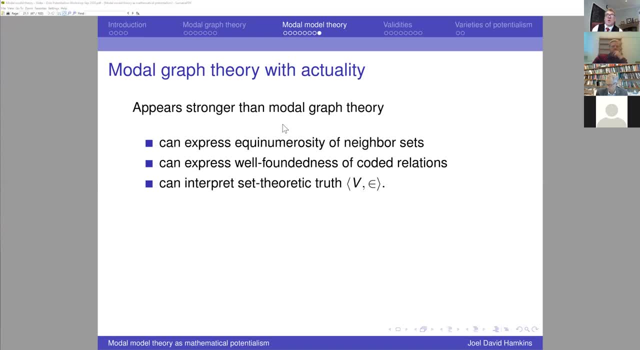 equinumerous neighbor set, or we can express the well-foundedness of coded relations. We can interpret full set theoretic truth in modal graph theory with actuality, But we don't know how to do that without actuality, And so it's a question whether actuality is expressible in modal graph theory. 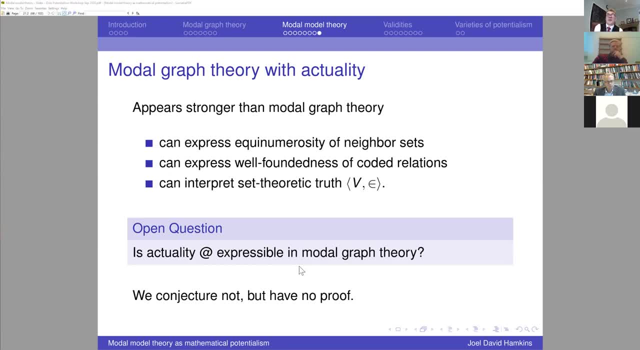 We don't know how to do it. I don't think it's true. I think that none of these things is expressible, actually, in modal graph theory, But I don't know how to prove that. Now let me come to these modal validities. 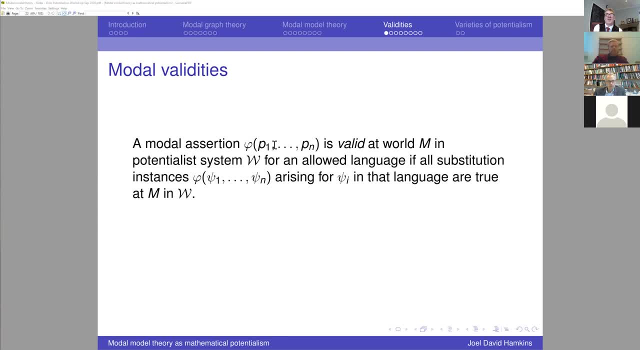 So let's look at this. So an assertion is valid at a world, So these are propositional variables here, If all of the substitution instances where you replace those propositional variables with assertions in the substitution language, are true at that world. So we're talking about validities, not with respect to a proof system. 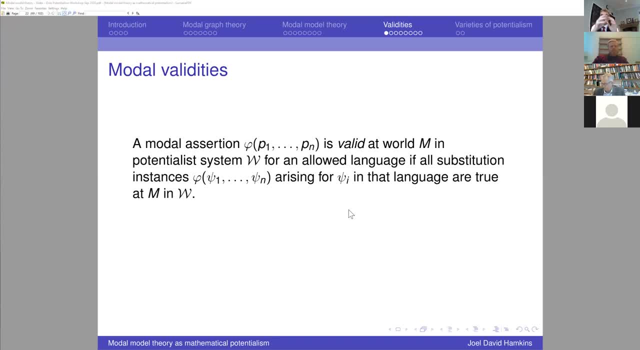 This is entirely semantic notion. We have this potentialist system, We have a world in that potentialist system And we're saying that a certain kind of modal statement about propositional variables is valid. Think of that statement as a kind of scheme, that standing in for all of its substitution. 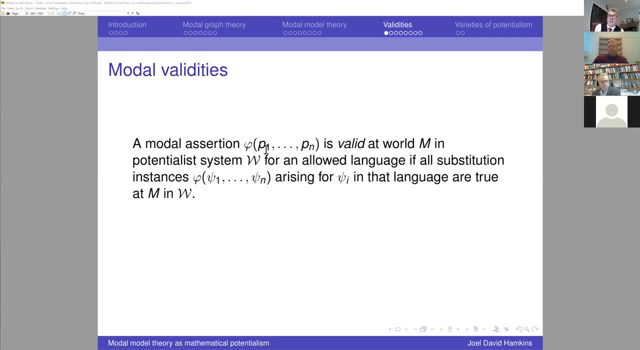 instances where the Ps are replacing the propositional variables. And also I want to emphasize that when we say something like S4.2 is valid at a world, we're not thinking of S4.2 as a logic, but as a theory. 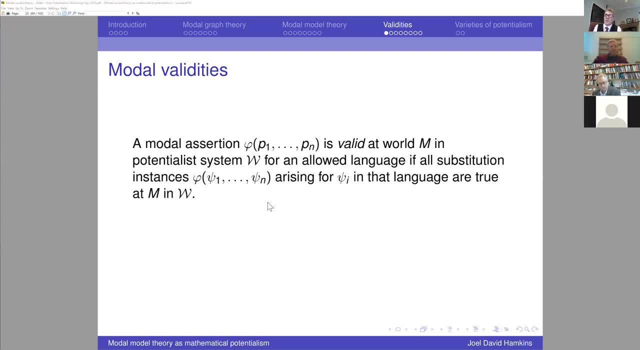 As a modal theory, Nearly as a set of propositional modal assertion, And the reason is that, whether or not a modal assertion is valid, it's often extremely sensitive to the language of allowed substitution instances, for example, whether parameters are allowed and because of this it doesn't interact. 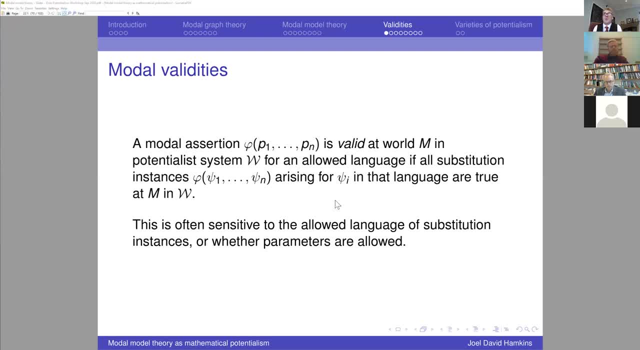 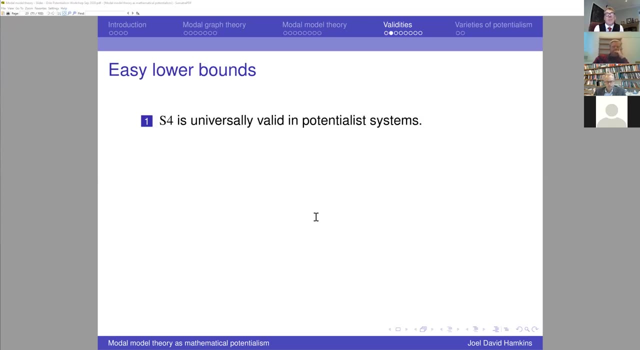 very well with the uh, with the rules of inference and the proof system, um, even though, for example, maybe we can validate s 4.2, but only if you don't allow parameters. if you do, then you don't get s 0.2 and we have all kinds of examples showing this very fine sensitivity. so this very easy. 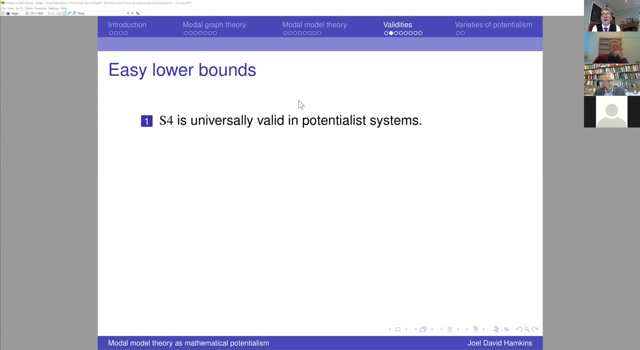 lower bound, some of which have already been mentioned. s4 is always valid in any potential system, as is the compost barking formula if you have a convergent potentialist system. so that means that if you have a world and it can see two other worlds, then there's a further world that they can both see, then s 4.2 is valid for sentencing. 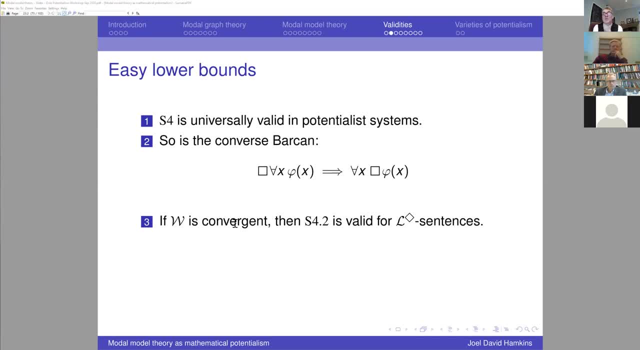 okay, but you need more than convergence. to get- uh, to get- parameters, you need amalgamation. and remember, direct extension is almost never convergent. it's embedded extension that is convergent. and then amalgamation is exactly the difference between convergence, because you have embeddings of the given world into two and then those worlds embed into the top one. 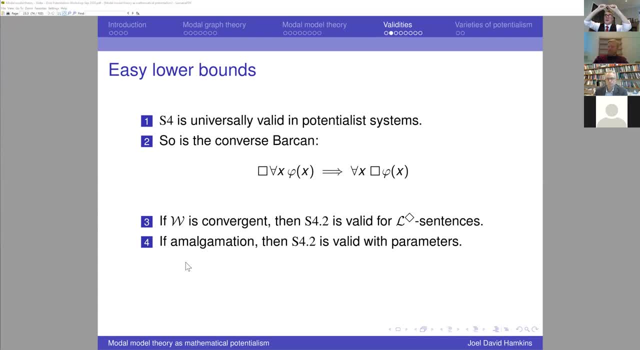 and amalgamation means that the data is not removed and then the data gets generated to diagram. commutes that any individual? if you trace the embeddings this way or this way, you end up in the same place. That's what it means to say: the diagram commutes, and that's. 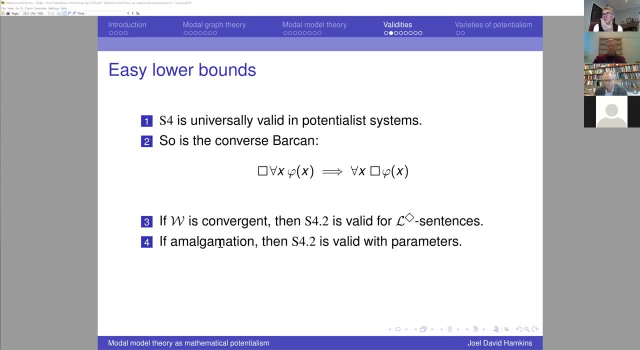 what amalgamation is. So if you have amalgamation, which you often do, then you get: S4.2 is valid, even with parameters. If it's linearly pre-ordered, then S4.3 is valid. Okay, now I want to emphasize that those are the easy lower bounds to show that something 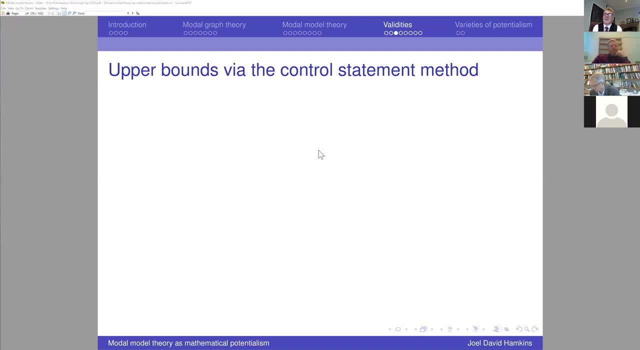 is valid is easy. To show that something is not valid is much, much harder. but we have this technology emerging in a series of papers over the past 10 years or so: the control statement method of proving upper bounds on the validities, And so we have these. 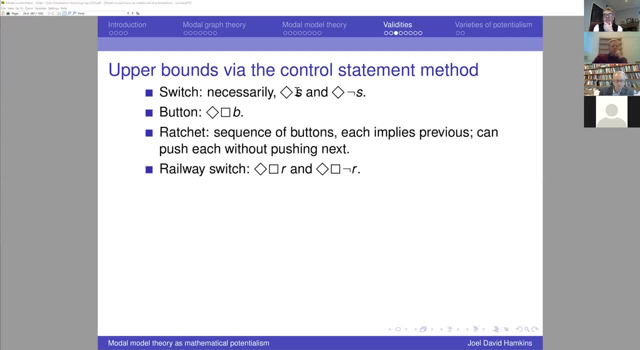 different kinds of control statements. So a switch is a statement which is possible and the negation is possible over any world, So you can turn it on and off like a light switch. A button is a possibly necessary statement, So you can make it necessary. You push the button. 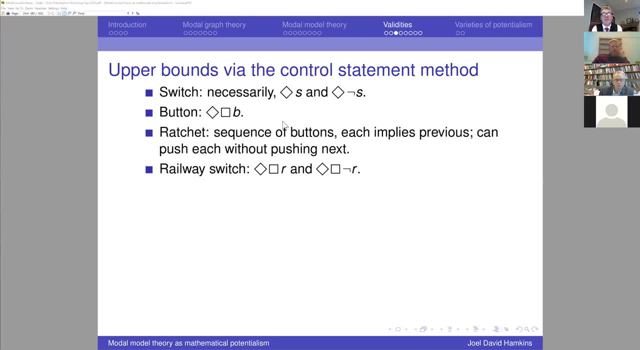 and you can't un-push it. A ratchet is a sequence of buttons so that you can push each next one without pushing the one after. So each of them implies the previous one. So it's this one. it's this unidirectional thing. you can push more and more and you can stop at any point. 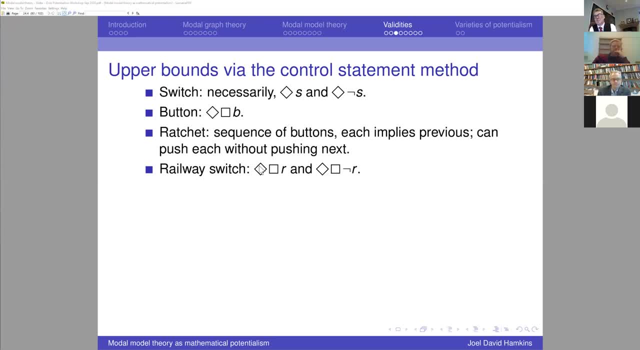 A railway switch is a statement R, which is possibly necessary, and the negation is also possibly necessary. So you're at the railroad tracks, right at the switch and the train is coming. You can make it go that way or you can make it go this way. 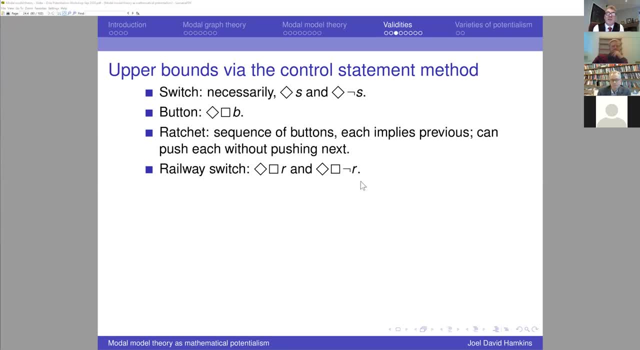 But once the train goes by, then it's all over. So you either made it necessary or you made the negation necessary. This kind of situation is, of course, fundamentally incompatible with S4.2.. This is a kind of S4 situation. 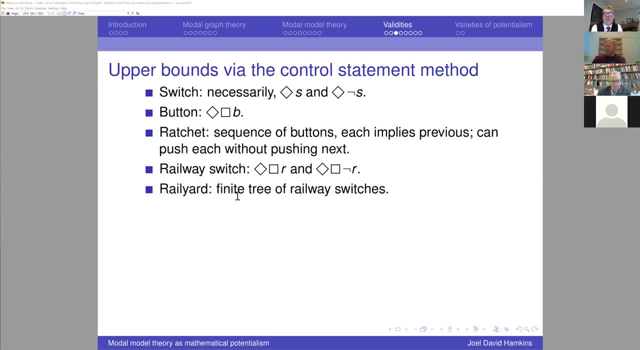 And then if you have a finite assemblage of these railways which is like into a tree, then this is what we call a rail yard, And the basic theorem is that if you have independent switches in a potential system, then the validities are contained in S5.. If you have 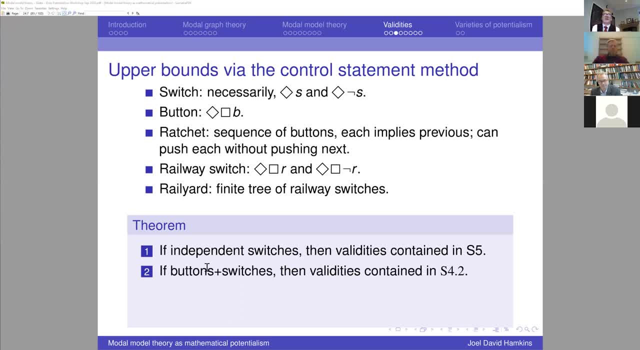 independent buttons and switches. independent means that you can control these statements independently. You can switch any switch you want without switching the other ones, and you can push any button without changing the switches, and so on. Then the validities are contained in S4.2.. If you have ratchets, then it's. 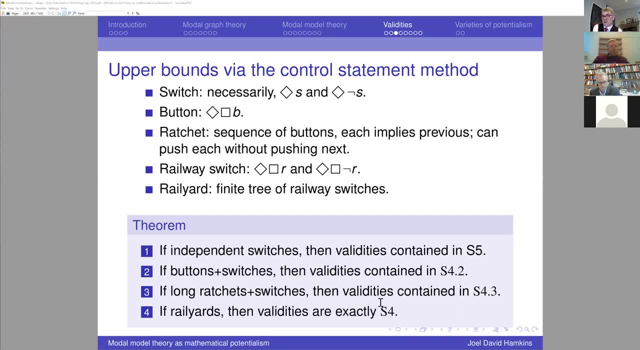 you know S4.3.. And if you have rail yards, then the validities are exactly S4.. So this is a much harder theorem than the previous observations that certain things are valid- And this is part of my interest in this subject of potentialism- is really to analyze. 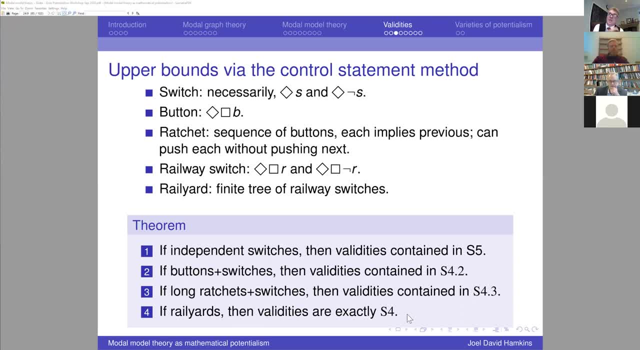 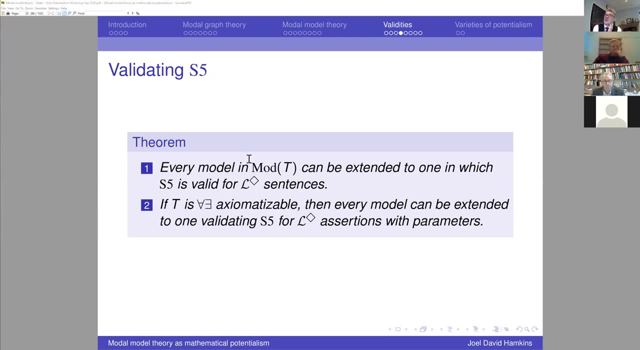 exactly what the modal validities of a given potentialist system are, And so we really need both sides, the lower bounds and the upper bounds. Okay, so right Now, if you have, if you're in mod T again, so the models of a given first order theory, say all graphs or all fields. 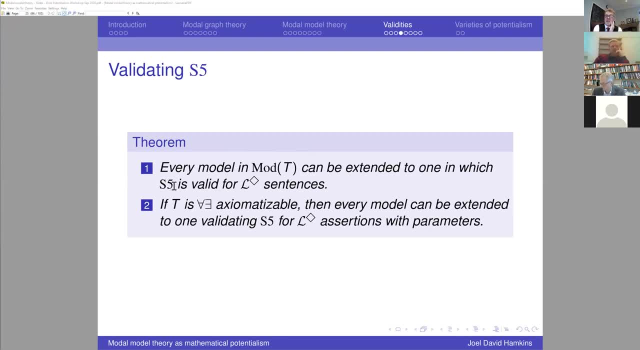 then you can always find an individual model in which S5 is valid. I'm not saying S5 is valid at every world, just that that world is valid. That's a model of the maximality principle. And if the theory happens to be Ae-axiomatizable- as many theories are, for example group theory- 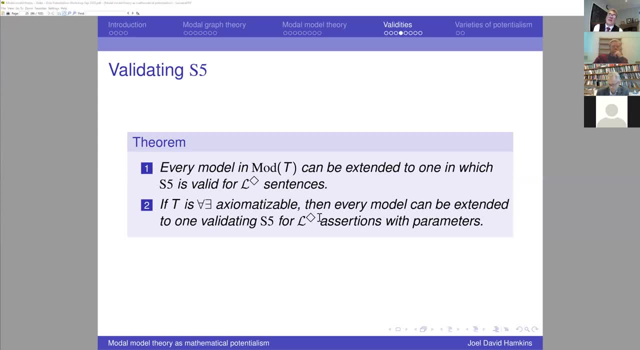 these are Ae-axiomatizable theory, then every model can be extended to one where you have S5, even with parameters, And these are both chains of models. argument because, as S5 is the assertion right that every possibly necessary statement is already true. 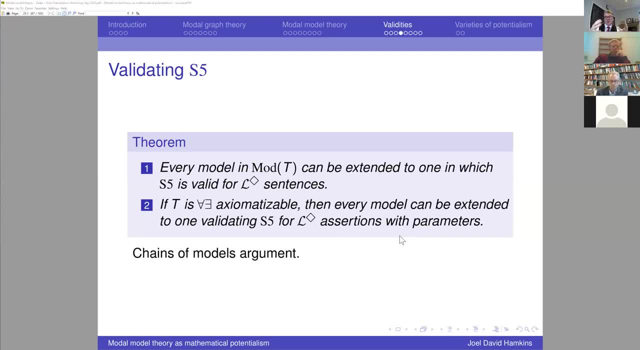 And so it's saying every button has been pushed. And if you have a model and it has an unpushed button, then you can make a bigger model where that button is pushed, In other words where that statement is necessary. And there you have an example of that. 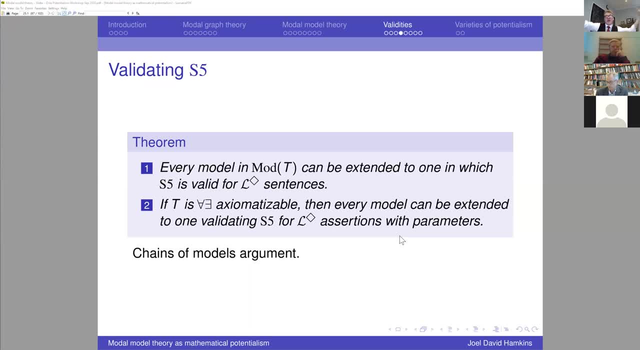 another one, then just make a bigger model, and if you just do that, then you're going to push all the buttons that could possibly be pushed and then you just need a bigger model on top of all those and that model. if it thinks something is possibly necessary, then all those individual models also. 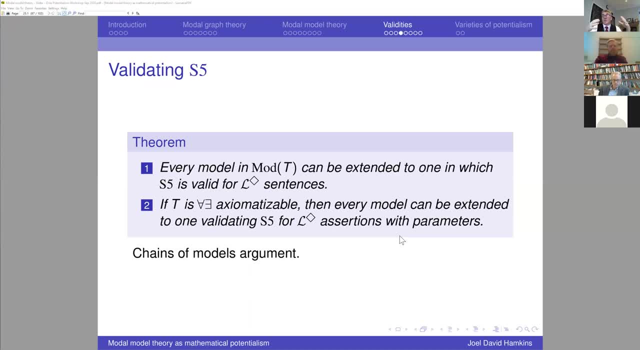 thought so, because they could have gone all the way up here, and so it must have already been pushed. you already pushed all the buttons and that's why you get s5 and the ae. aximatizability is just used to know. it's a kind of continuity of the chain. it's equivalent to saying that the 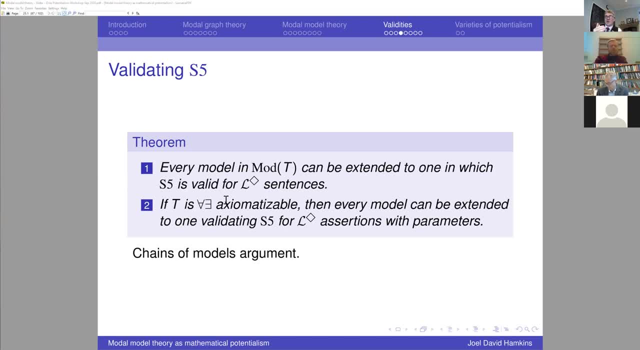 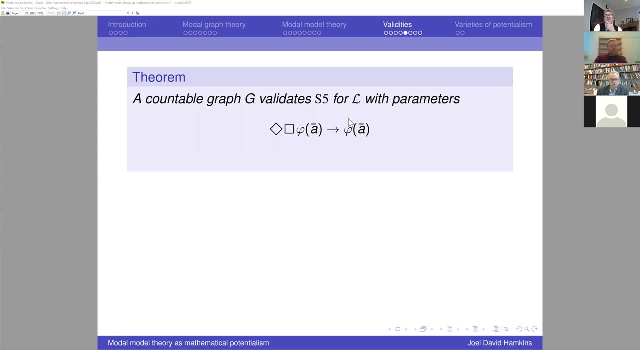 union of a chain of models of t is also a model of t, and so you didn't introduce any new parameters when you went to that bigger model on top, and that's why you get s5 for the parameters in that model, because you didn't have a new one. so it turns out that, let's see, i want to pay attention. 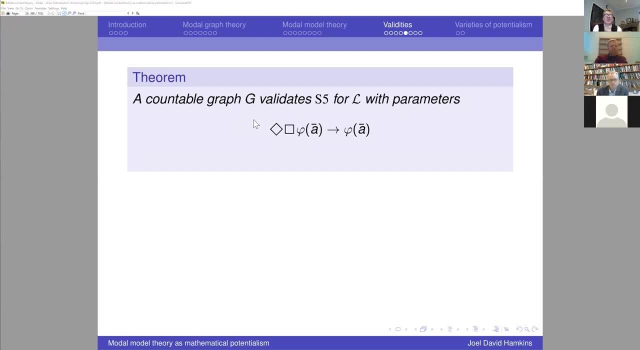 to the time. so we have some interesting results about model graph theory. a graph validates s5 with parameters, so this is the s5 axiom. possibly necessary statements are already true if, and only if, it's the countable random graph, which is a very natural countable graph to be looking at. and uh, and it validates uh. 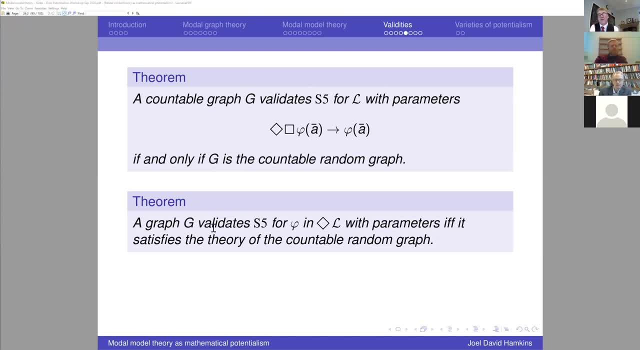 in general, this is a countable graph. an arbitrary graph validates s5 with parameters. just in case, it satisfies the theory of the countable random graph, which is called the finite pattern property or the alice's restaurant property, if you put that um. so a graph validates. 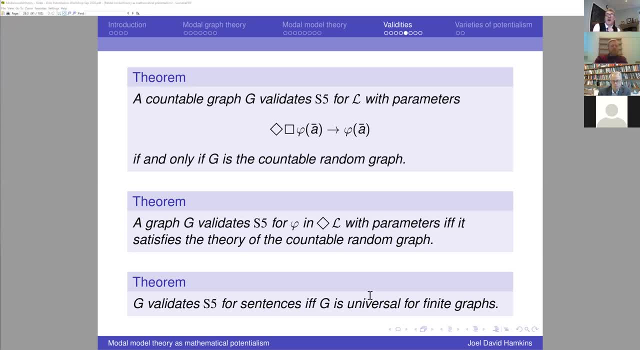 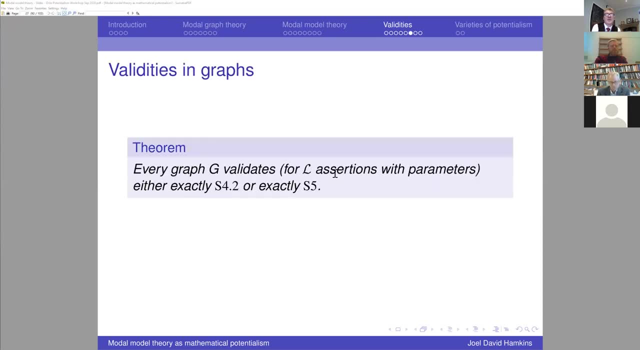 s5 for standards is only just in case. it's universal for finite graphs, meaning that for any finite graph there's a copy of that finite graph inside g, um. so these, all those themes are really generalized by- oh, i see, um. so a graph g validates always either exactly s 4.2 or 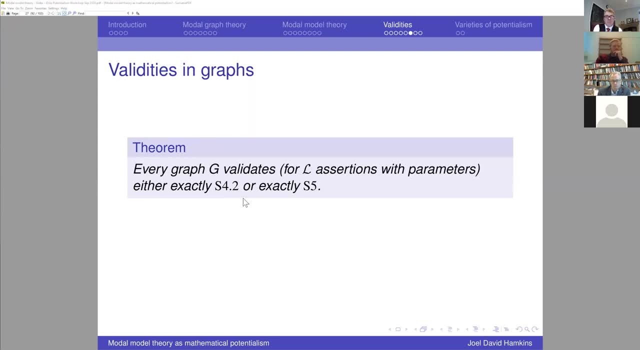 exactly s5. okay, um, there's no other possibilities. if you're talking about assertions with parameters and the reason is that, uh, if it has the finite pattern property that characterizes the countable random graph, then it will satisfy s5, and if it doesn't have the finite pattern property, 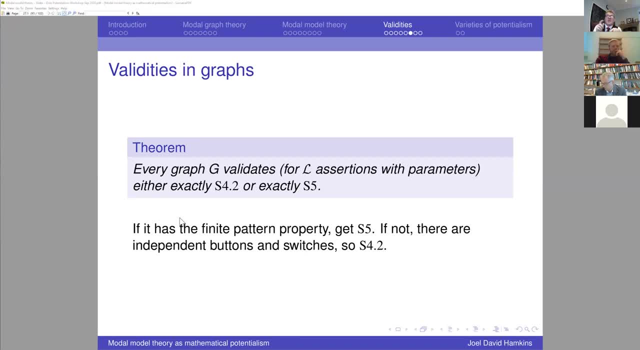 then there's a finite instance of that property that fails and you can use that failure to generate buttons and switches which show that only s 4.2 is valid, but meanwhile s 4.2 always is valid because it has an alternation and therefore you get exactly s 4.2 or exactly s5 in any graph. 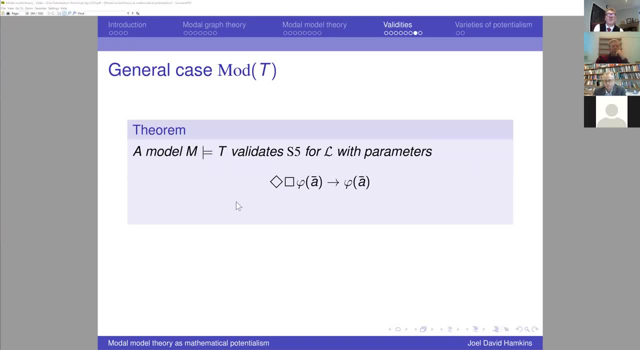 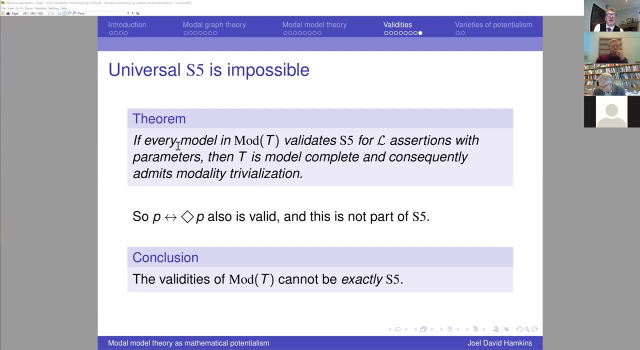 so i guess i'm almost out of time, so let me just skip this part here and mention two more things. so this we just proved a few weeks ago: it's not possible that every model has s5 unless it also has more. you can't. you can't always have s5, because if, if, s5 is valid. 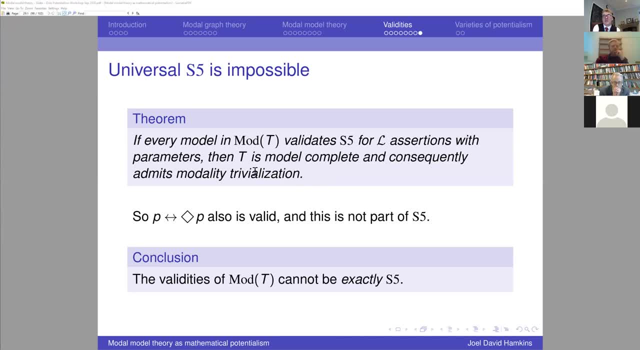 in every model, then you must have modality trivialization, and so you get the trivial modal logic being valid, and that's not of course in s5 validity. this is strictly stronger than s5. so if every model has s5, then in fact the modal logic is trivial. so they can't be exactly s5. 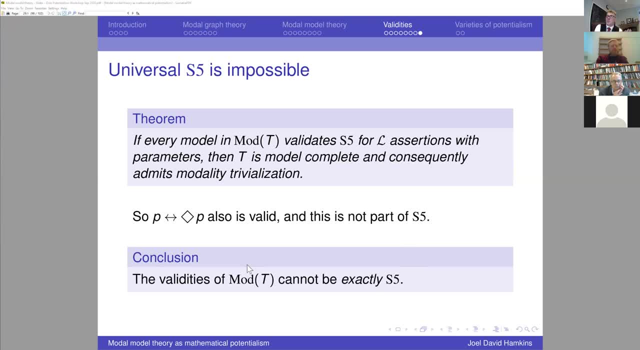 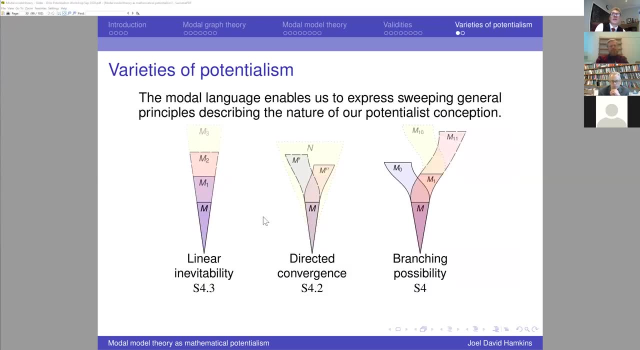 ever. this is in mod t. of course you can present other potentialist systems that aren't mod t, in which you have executives. so let me close just by mentioning, in keeping with the theme of the workshop this, varieties of potentiality. so i think it's important- i mean, the way i approach the subject of potentialism is 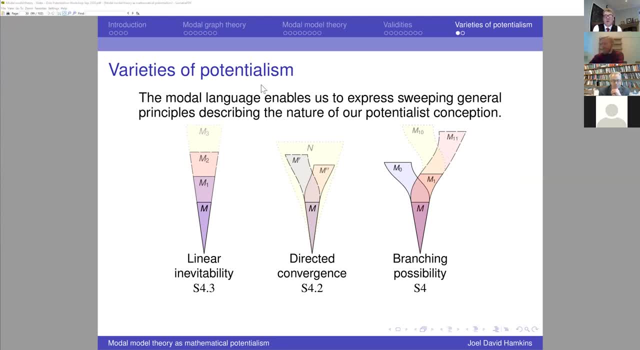 a kind of from a semantics point of view, from the ontology, rather than from looking at proof theory or looking at principles or statements that you want to be true for potentialism. we look at: well, what are the ontological commitments of your conception of potentialism? What are the worlds like? And then, when you understand what they're like, 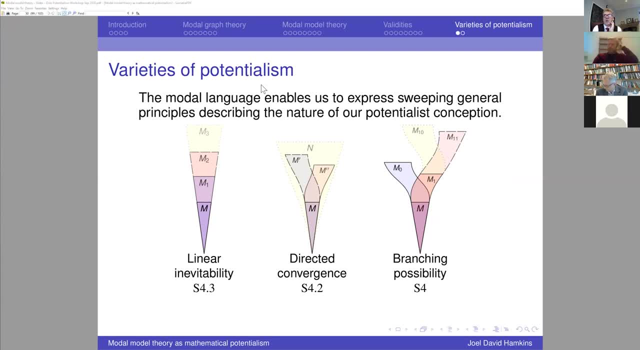 then that's going to lead you towards which modal principles you want to adopt. And if you have a picture of potentialism in which there's a linearly growing hierarchy of possible worlds- and to be possible just means to be true in a taller one- then this is what I call. 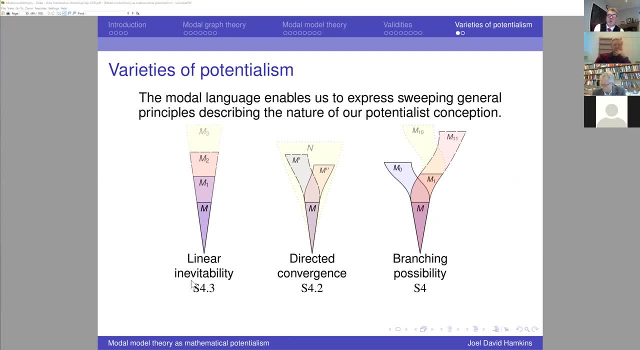 linear inevitability And you're going to see that S4.3 is valid always in such a kind of picture. So this is true, for example, in rank potentialism and set theory. If you have a kind of understanding of potentialism that well, maybe temporarily you can extend in different directions, but if you go, 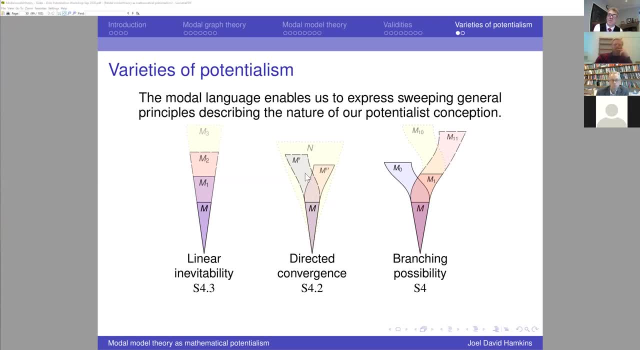 further, then you're going to bring those two, you're going to encompass those two inside a larger model. So this is the directed or convergent conception of potentialism. Then this is what leads you to S4.3.. But there's another, more radical kind of potentialism, what I call radical branching, or 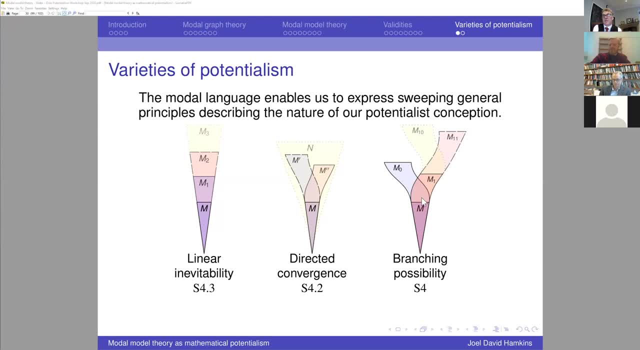 branching possibility, namely where the kind of potentialism that you have has fundamental choices to be made. So if you're living in a world M, then maybe you can extend to M0, or maybe you can extend to M1. But if you go to M1, then you can never extend further so as to encompass what you. 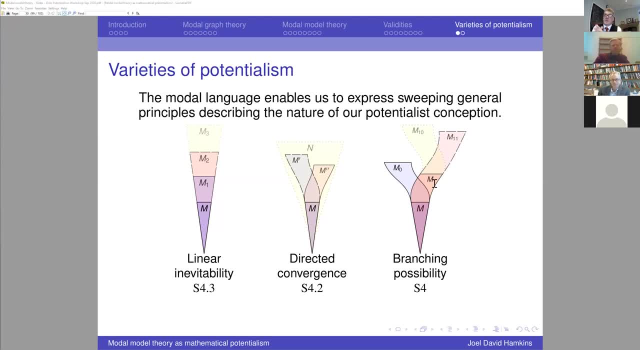 might have had. So we have many potential systems exhibiting this. For example, top-extensional potentialism in set theory, Hugh Woodman and I proved has this form. And also end-extensional potentialism in set theory has that form. Cameron Williams and I proved that. And in arithmetic I proved that. 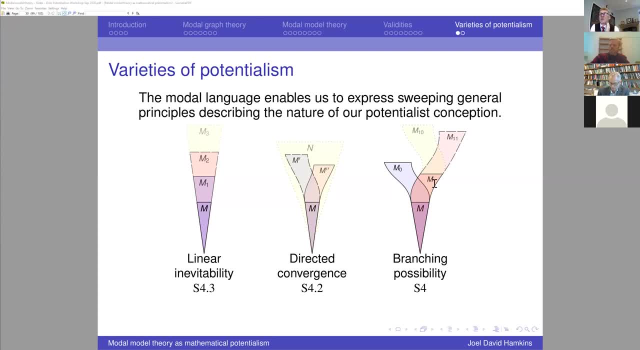 top-extensional, end-extensional potentialism in models of PA has this form, And in all these forms you have really only S4. And this has to do with this, This radical branching. it's like a railway switch here. Which way did you go? And I've mounted the. 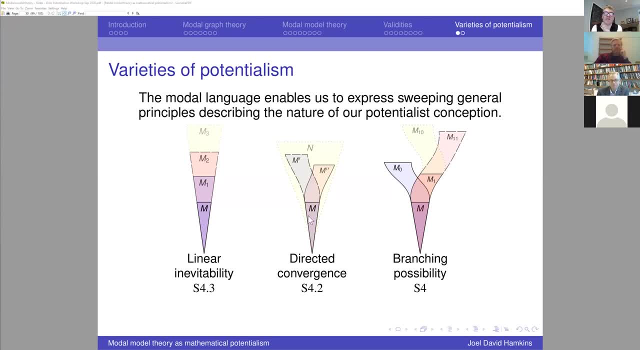 criticism that these forms of potentialism are what I call implicitly actualist, And the reason I view them that way is that the universe fragments in the ontology of the potentialism are converging to a limit model. This, for example: maybe this is something like what ultimate V would be in Sam. 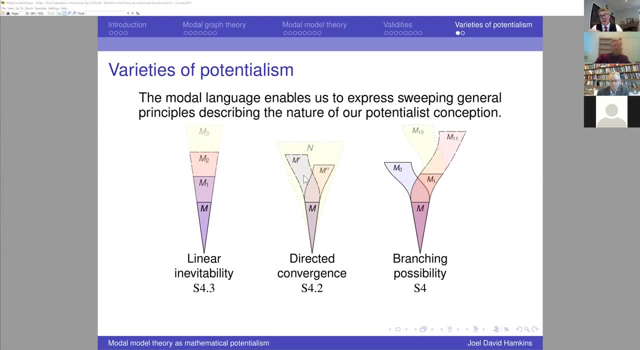 Roberts' talk, And without adding any new objects or structure to the ontology, but only sort of taking a limit of what is already there. for the potentialist, you have the limit model, And that's a sense in which that kind of potentialism is implicitly actualist, because the difference between saying well, the universe actually 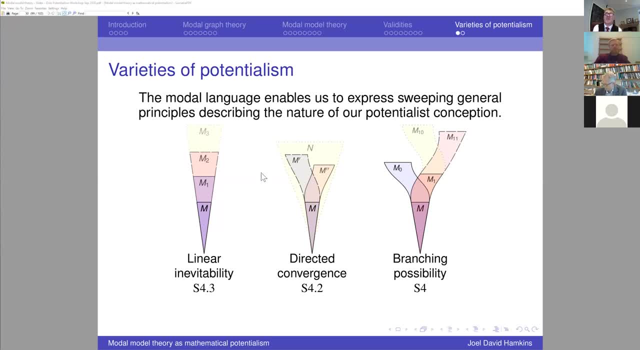 exists or it doesn't is a difference that doesn't seem to matter In any way, because we have the potentialist translation. we can talk about truth in that limit model, even if the limit model doesn't exist in our ontology. Whereas in this radical branching kind of potentialism there is no limit model And it's a fundamentally different kind of potentialism where you don't know what's going to be possible yet. you have to wait and find out what comes into existence in order to discover what the possible truths are. 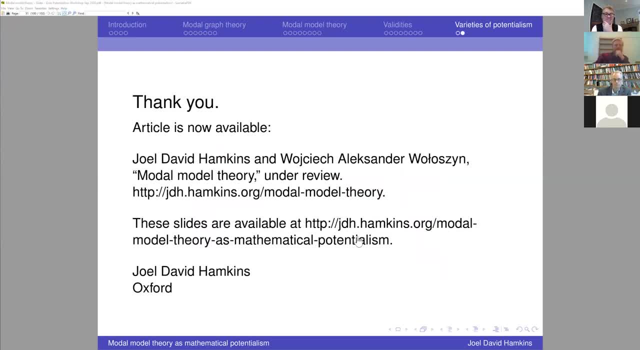 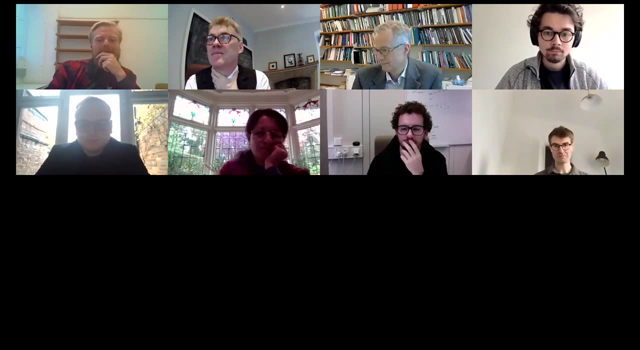 Okay, so thank you very much. Thank you, Joel. So we have some time for questions, so people can just write in the chat And I see Øystein has. yeah, you can start off, Øystein. Thanks Joel. 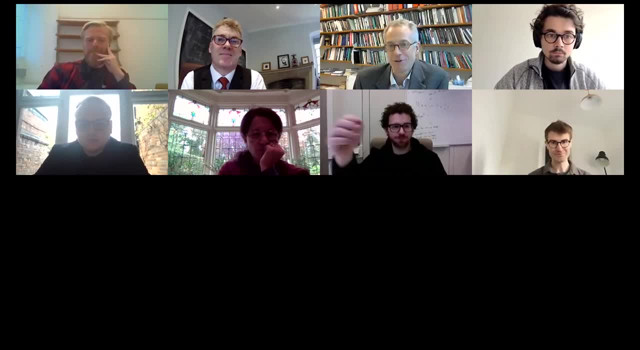 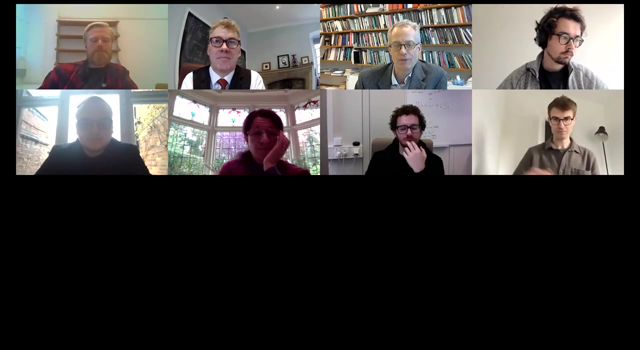 That's full of fascinating material. I'd like to pick up on the implicit actualism, Sure, From the very end there. So, yeah, there is something, some common ground with the actualist, for sure, And I think that's very nicely reflected in what I like to call the mirroring theorem. 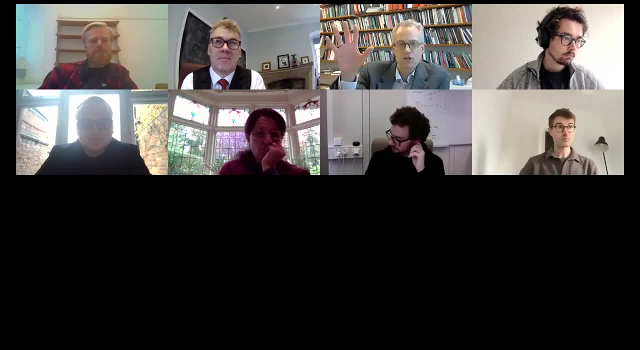 So the fact that you can then use the potentialist translation and recover ordinary classical first order logic. So for the purposes of the first order theory, the mathematics and logic that you get is exactly what the actualist would get. But once you go to higher order or non-first order settings, differences do emerge. 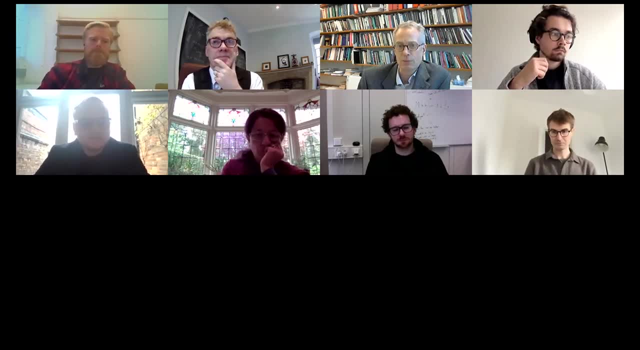 which is why I wouldn't see this as a complete actualism. So look at collections understood in some combinatorial sense, so that the collection presupposes each and every member of the collection, So say pluralities or combinatorial sets. Then for the potentialist to have a combinatorial collection, 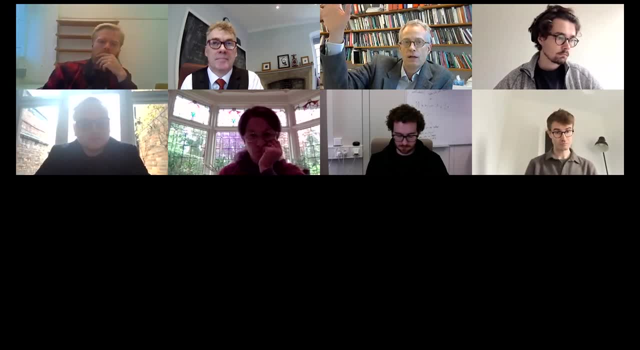 you've got to have each of the members at the relevant stage. And since there's no stage where you have all of the members, then you haven't got, say, naive, plural concepts, Plural comprehension, or you haven't got a universal set. less surprisingly, 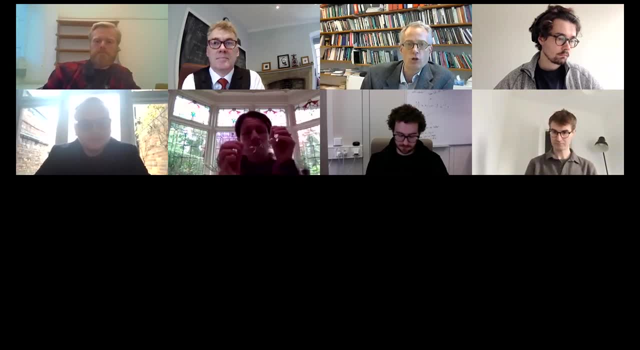 So differences emerge once you go beyond first order logic, is what I would want to say. Right? Well, let me respond to that. So there's different ways of understanding the sort of second order logic in the potentialist setting. I mean one way is that: well, when you have a second order quantifier, 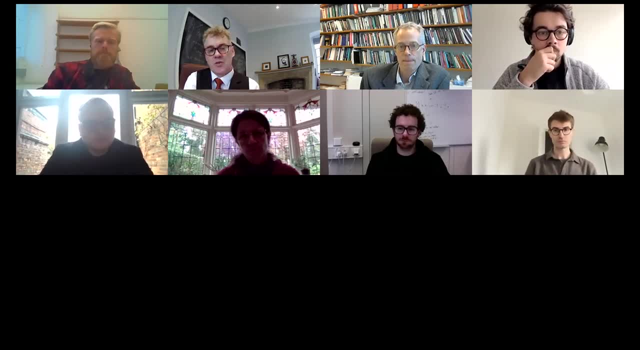 I mean, one has to be very clear. I think If you have a second order quantifier, then if you use it at an actual world in your potentialist system, are you just quantifying over the sub-collections of that object? 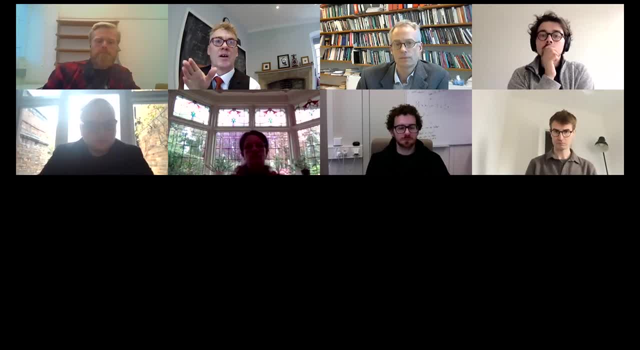 This is like Sam's plural quantifier. I think That's how he was interpreting the plural quantifier in his version. Okay, but another way to do, and with that understanding of second order logic, then I don't think your objection applies. 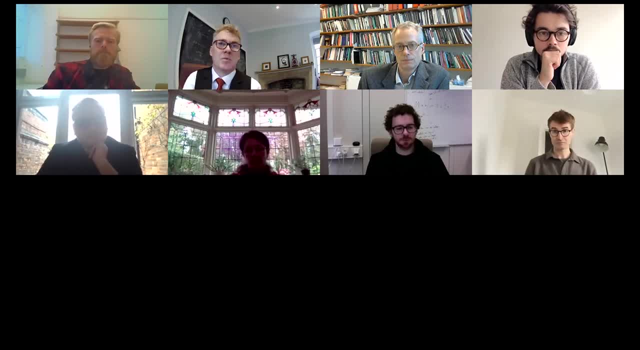 I think that if it's convergent, then it's still explicitly- I mean it's still implicitly- actual, Because we can- all those second order quantifiers can be viewed as just basically second order quantifiers over the over the limit model. 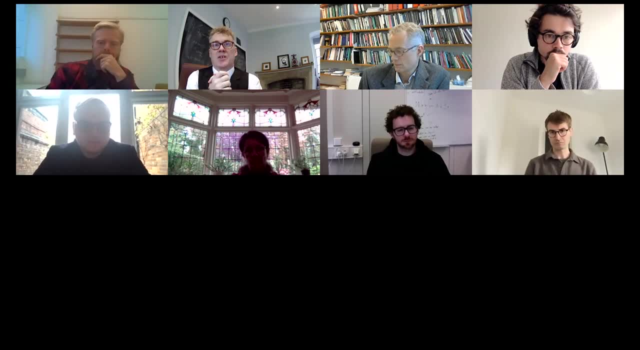 But if you have another more robust version of the second order quantifier which would go beyond what Sam was talking about, where you're quantifying over classes of possible things like, for example, I might and you can do this with plural quantifier, class quantifier. 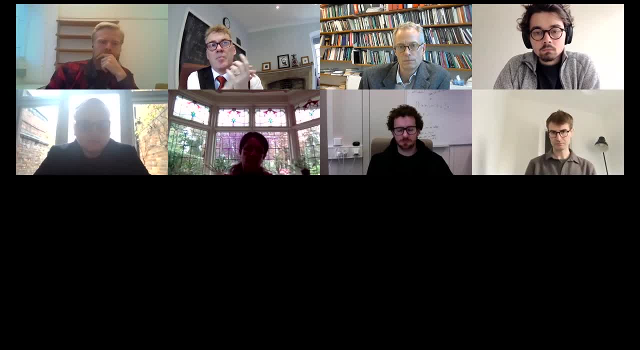 To me those are basically the same thing. if I consider, say, all the possibly all the possible red things, That's not a plural quantifier in Sam's sense, But it's a second order quantifier in this more robust sense. 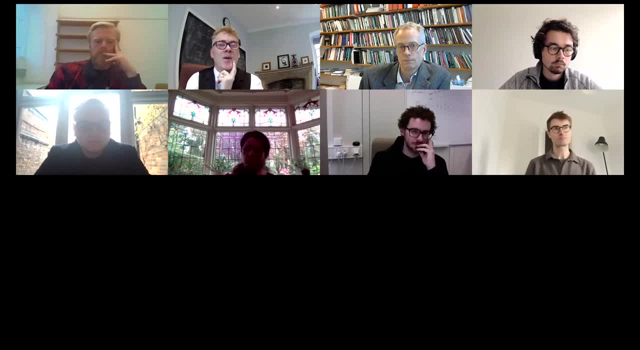 And I would say, well, look, if you are serious about those kind of second order quantifiers, then you shouldn't be a potentialist That's talking about this enormous object. that's way beyond. I mean, the potentialist is saying, well, look, I can't really promise about the things that exist way up there. 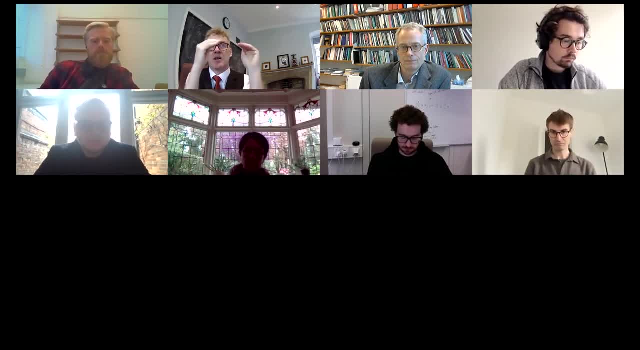 I'm only going to take the actual things and then a little bit more, and then a little bit more. And for such a kind of potentialist to say: but I also want to talk about these classes, of all the possible things and so on. 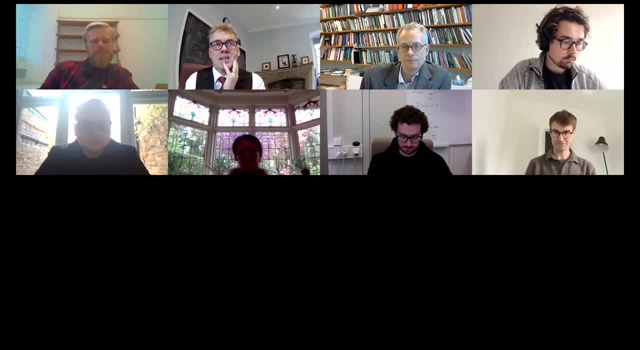 there's huge tension between that kind of interpretation of second order logic and potentialism, And so I don't think that one can ground an objection to one kind of potentialism or another based on that kind of combination of potentialism plus enormous classes being part of the ontology. 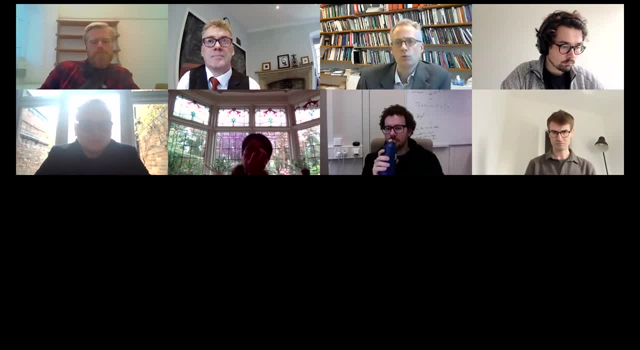 Yeah, I certainly agree with the last thing you said. So if you want to be a potentialist, if you want to be a potentialist in any meaningful sense, then the second order entities- just to call them that- they too need to be generated in some sense. 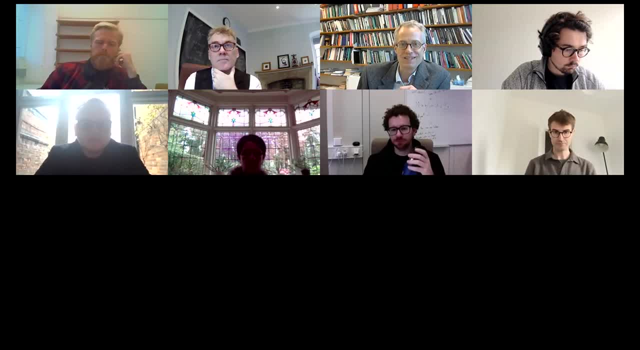 since otherwise it's unclear in what sense this would still be a potentialist. So if you wanted to have second order entities that grow as you consider ever larger worlds, then those entities would have to be generated in some other way So they could be understood in a property-like way. 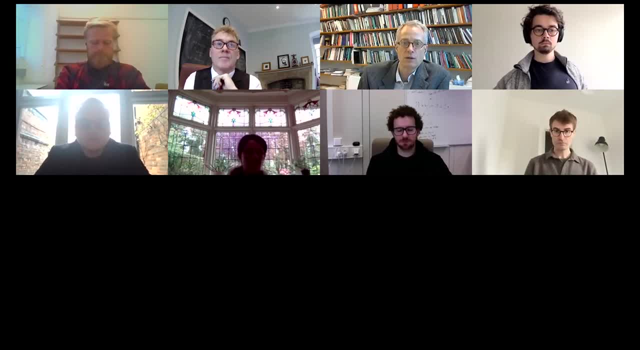 where you give maybe a predicativist account of how these properties are generated. but you've got to say something, since otherwise I think it's connected with Neil's question about, say, Kelly Morris or Gertle Bernays set theory. 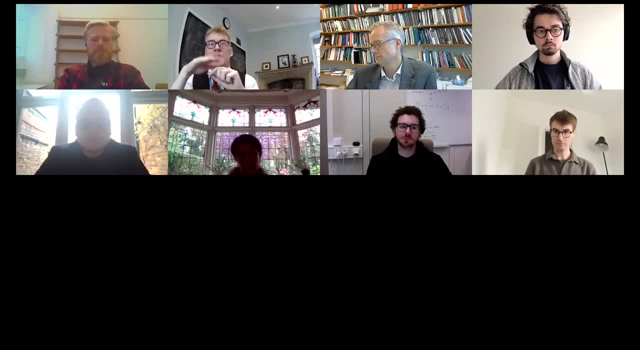 because you're talking about. well, if I have an actual world, a model of set theory and I've got classes there, then when it's extended, then those individual classes should also extend into classes of the extended model, And then it's something like what you were just describing, I think. 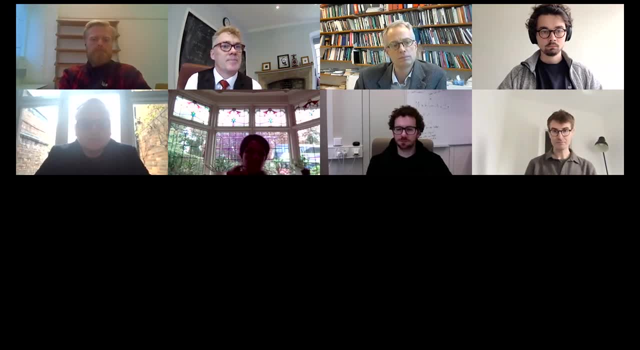 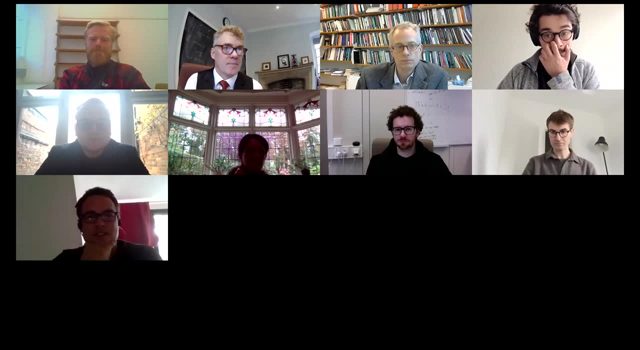 Great. So then the next one is Neil. Oh thanks, This is really really interesting stuff. My question is: I mean it's maybe a little speculative, but have you looked at all at how or if this can be used to deal with more kind of model theoretic questions? 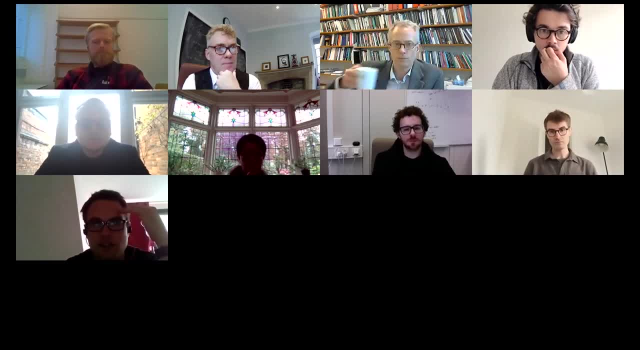 about, say, classification of different theories? I mean, you have this nice, nice result early on, that model completeness and, if I recall correctly, S5 are linked. Are there other model theoretic things you can classify using the modal logic? 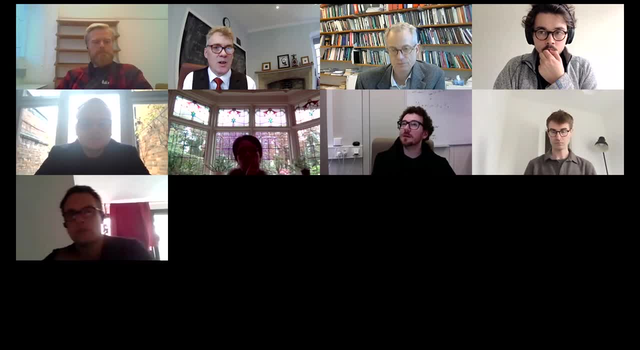 Yeah, so that's exactly. our goal is to sort of start doing modal model theory. So that's the title of the paper. It's just on the archive. I mean we just put it on the Math Archive a few days ago, So the paper's out. 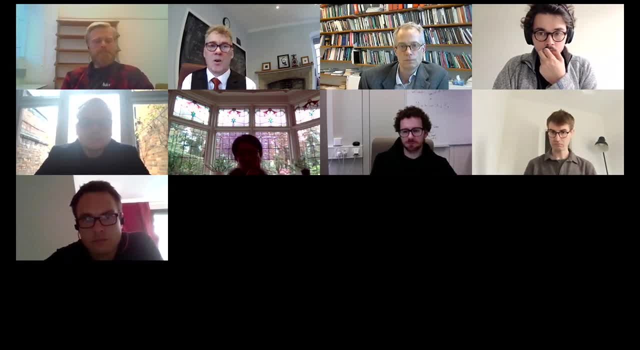 And that's exactly what we're trying to do is figure out to what extent, for example, we can show compactness doesn't hold in the modal language, not even for the Diamond-Dell case. The Walsh ultra-power theorem doesn't work in the modal language. 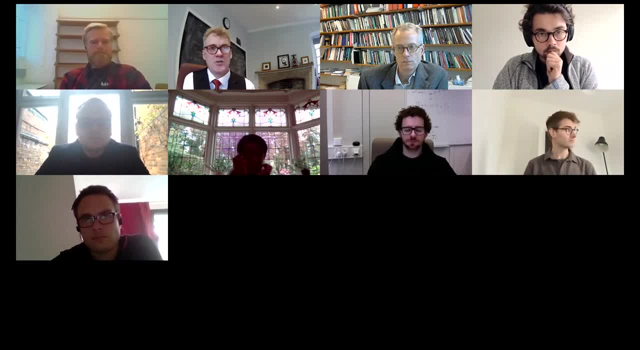 A theories model, complete, just in case it has modality trivialization. It wasn't S5, but modality trivialization. Oh sorry, Yeah. Yeah, that's right, And we have a collection of results along those lines. Also, the sort of definability of these cardinals is connected with the idea of 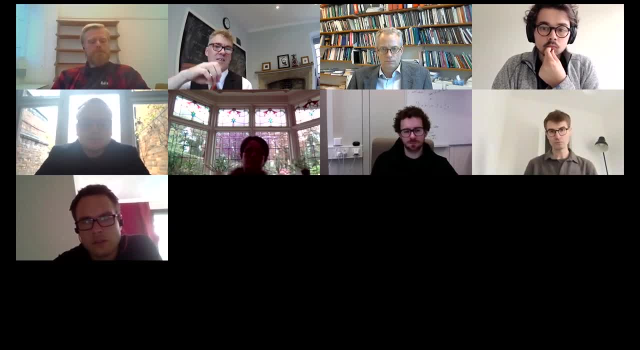 looking at, say, the Hartog number, the Levenheim number of the language, And we're trying to figure out exactly what those cardinalities should be. So the full modal language of graph theory can express these enormous cardinalities, And so we're trying to find out, well, what is the bound exactly? 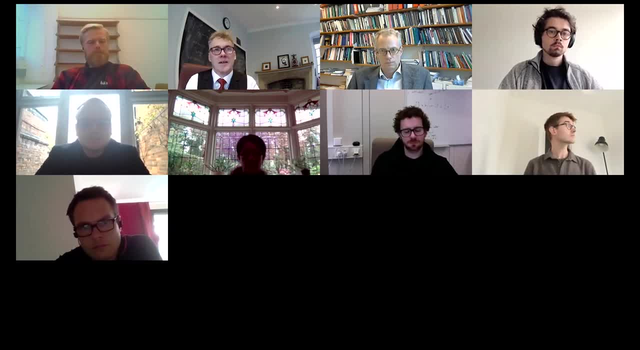 And how does it relate to the other cardinalities that come up in model theory? And also, for example, Wojciech in his dissertation is looking at fields, So a field in the context of all fields. you get S5 if, and only if, you're algebraically closed. 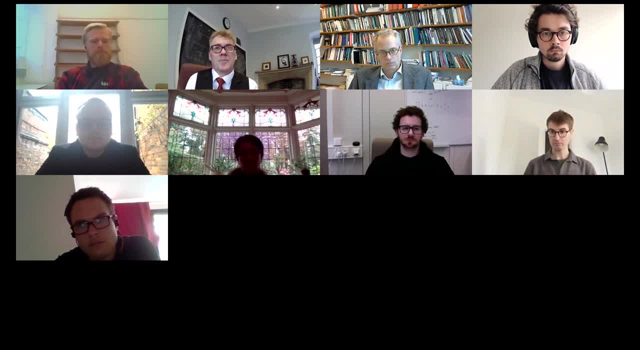 which I thought was a kind of nice result, And S5 for sentences if, and only if, you contain the algebraic closure of the prime subfield and with parameters, then it should be fully algebraically closed, And so we have different results along those lines. 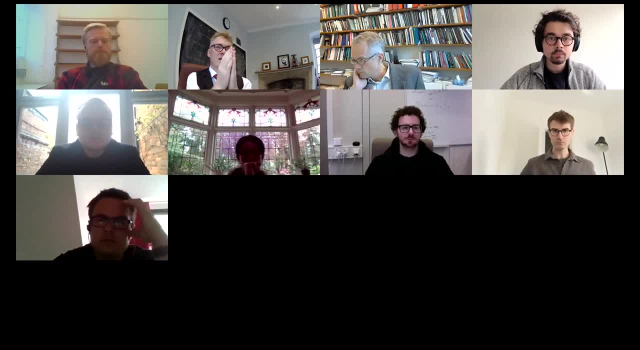 So we look at, say, linear orders. How do you want to extend one linear order to another? Well, you can extend it just like this: You can extend it as a suborder, Or you can extend it by adding new stuff on the ends only. 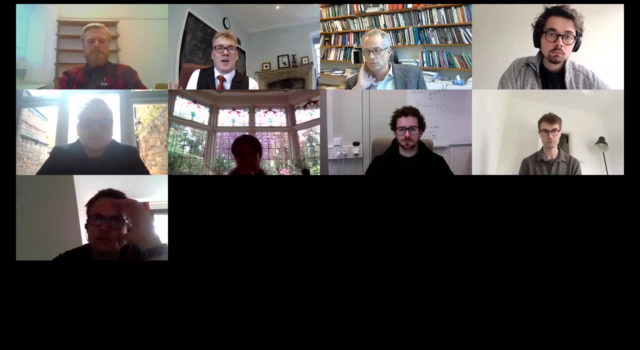 Those are two different potentialist conceptions of potential linear orders, And they have different features, And so this is the kind of project. I suppose, though for a lot of kind of things the model theorists look at, this is not going to apply. 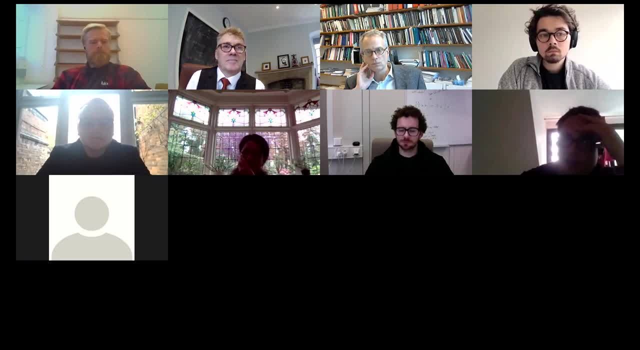 So, for instance, if you think about something like strong minimality, the theory has to be complete here, So it should be trivial, Right, But this still has this. I mean just naively thinking this somehow has this modal flavor of building things up for a lot of the models. 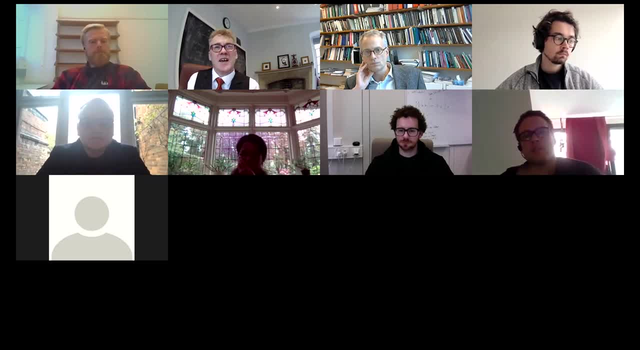 and things like that. I agree. I agree with that. So we're looking at mod T when T is complete, And of course then the Diamond-Dell theory is also determined. All the models have the same thing, But it's open whether that's true for the full modal language. 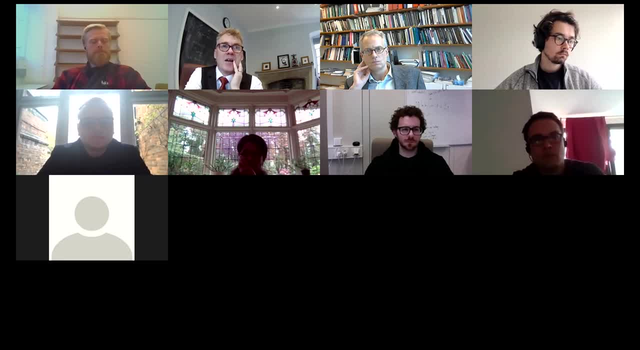 Ah, okay, You don't know the answer to that, Yeah, So there's quite a lot of open questions. Maybe some of them are easy, I don't know. I invite anyone to step in, Cool, Thanks, Thanks very much. 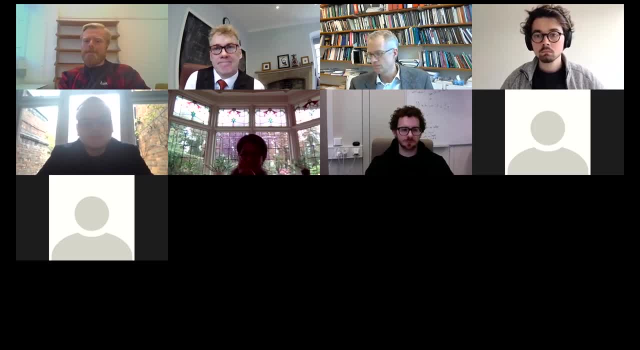 Good, So then Sam next in line. Yep, Thanks, So I wanted to. I've been thinking about this a little bit and I wanted to get your opinion on it. So on this divergent potentialism, right, Right. 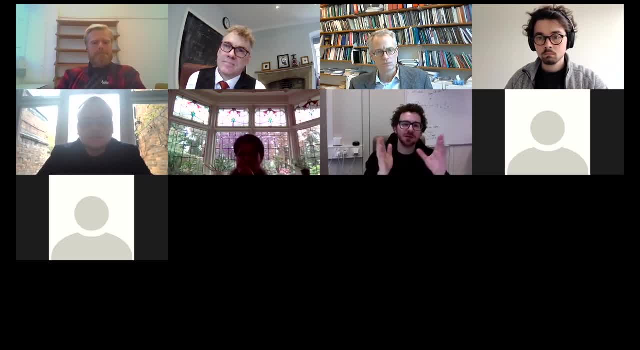 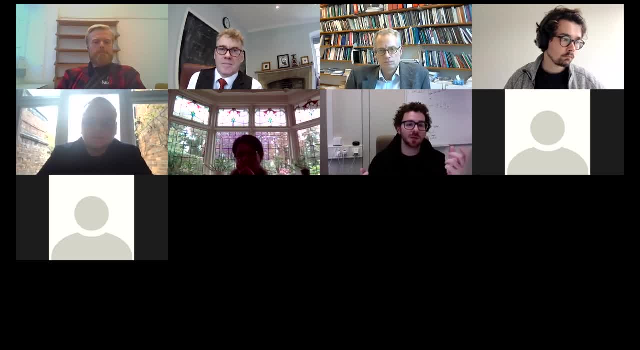 uh, uh, two generics over the same partial order that can't be combined right. One. Yes, Together they together, they code a uh, you know, uh uh. the claim that the universe is countable. the ordinals are countable. 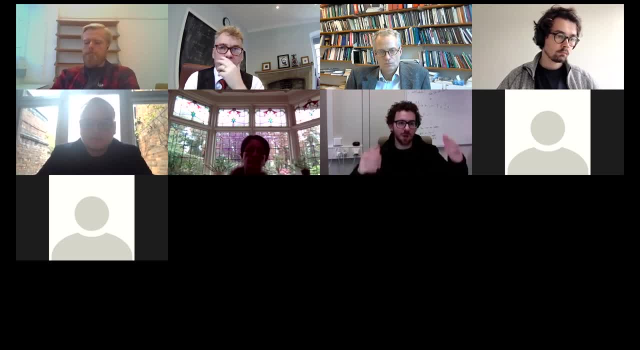 whatever, Each is okay on its own, but together they're not Okay, And that would be one of the instances where we can't combine worlds. Okay, And so, Actually, in that case, though, I mean, I have a paper actually about exactly that- non-amalgamation result. 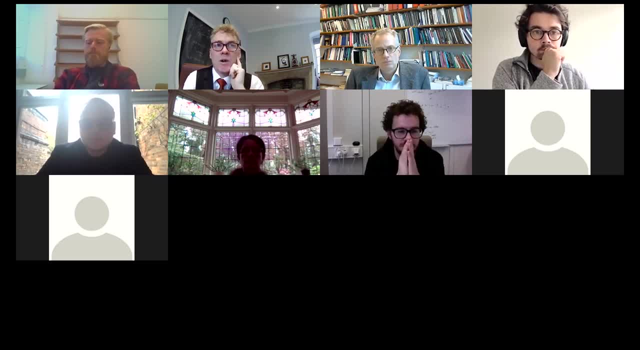 And in the modal logic of forcing, you do have S4.2 is valid even though you don't have amalgamation. Yeah, Right, Right. So that's what that shows. Yeah, Yeah, No, absolutely So. 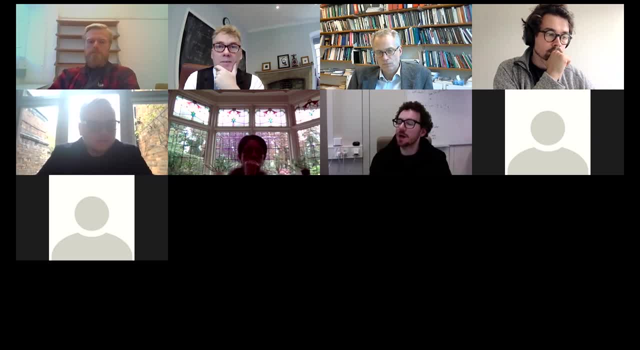 so, so you still get the, you can still get the. uh, the behavior without the, without conversion, Sorry, But but the the thing I was interested in is: this is: like: suppose you, suppose you want to go divergent? 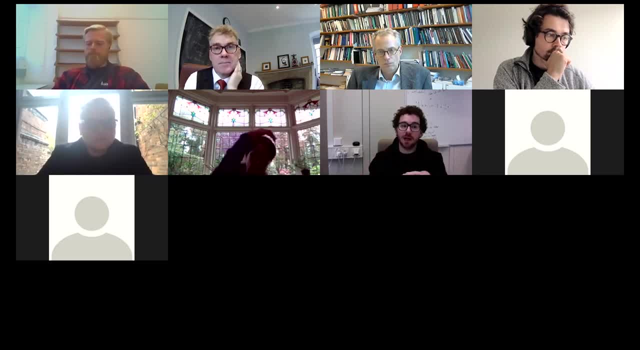 but you're also really committed to the modal collapse principle And you want to read it in the in the plural way, And so, in particular, you're going to think that there is a plurality corresponding to the union of those two generics. 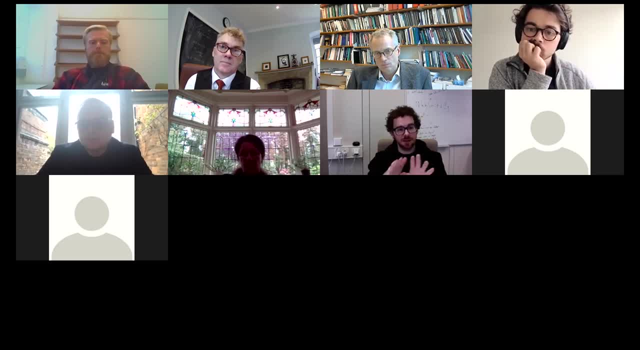 Um, and that plurality can't form a set in in that divergent structure, Um. so if you want to go divergent and you're committed to collapse, then the standard models of these divergent systems like just the generic universe over. 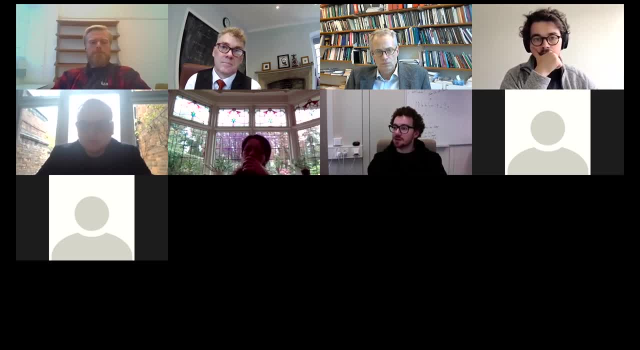 over M. um, multiverse over M is not going to be a good model of your, of your view, And I wonder what you? I mean, I'm not sure of the model you say. well, that's you know. 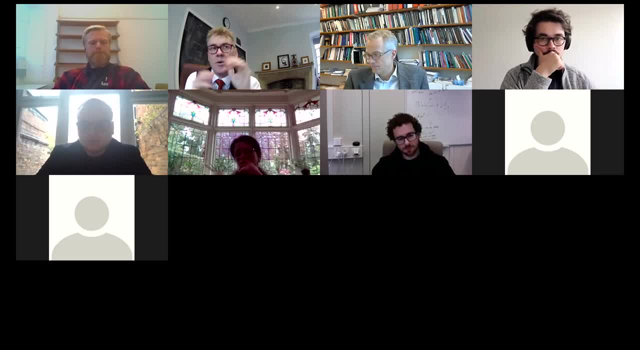 if you look at, if you look at models of set theory, or even just countable models of set theory under end extension, Yeah, Um, then you have only S4 and it and it has radical branching And this is a consequence of the universal algorithm. 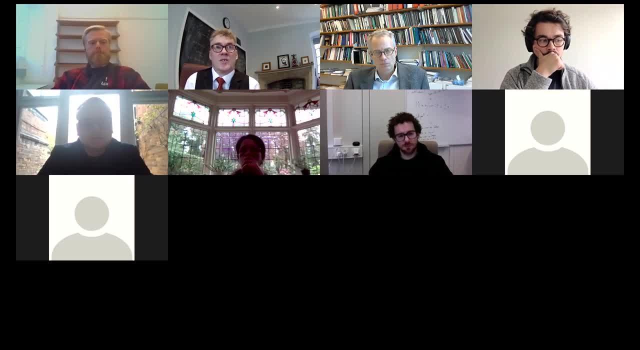 Uh, there are these Sigma one. there's a Sigma one definable sequence, a kind of Sigma one definable finite sequence. that can be anything And once you extend it to make the first element of that definable thing start with you know. 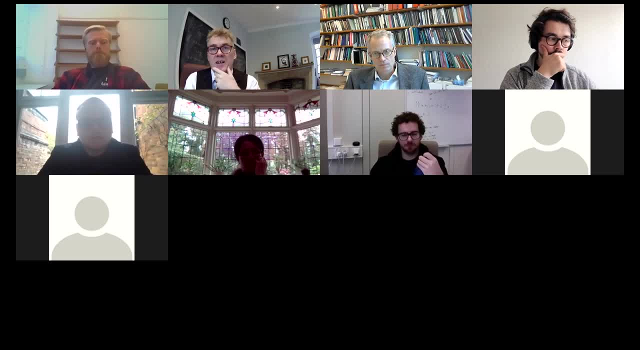 a certain set, then no further extension is going to make it start with a different set. but you could have had it start a different way. That's the kind of fundamental branching. So it's connected with these universal algorithm results. Yeah, Um. 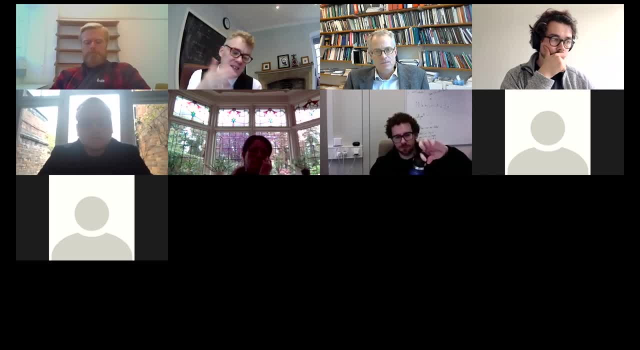 and even though, um, well, I mean okay. so in this, in this amalgamation result that you were just talking about, say, countable transitive models have sent through, then in my paper with Austin we we considered that case. 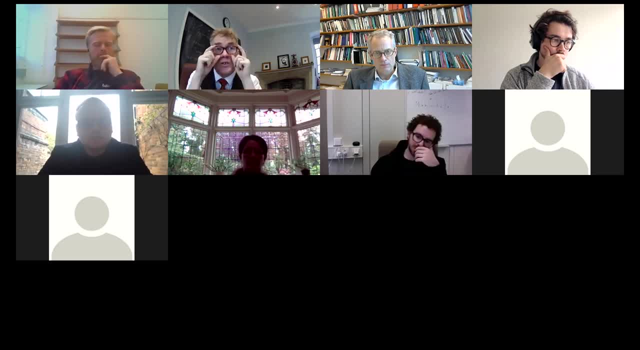 uh, and, and you do have S4.2 there and the limit model that you're converting to, so they can get taller and they can get wider, because they're just countable transitive models, So you can force over them and you can also make them taller and they. 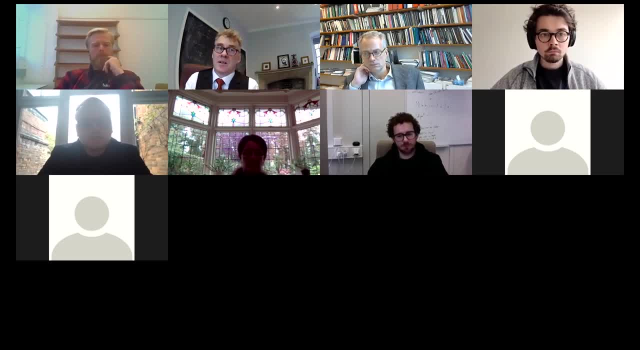 they are converging to a limit model, the ultimate V in that case. but it's not a model of CFC, It's, and it's not a model of the power set. It's. it's the H omega, one of the ambient set theory. 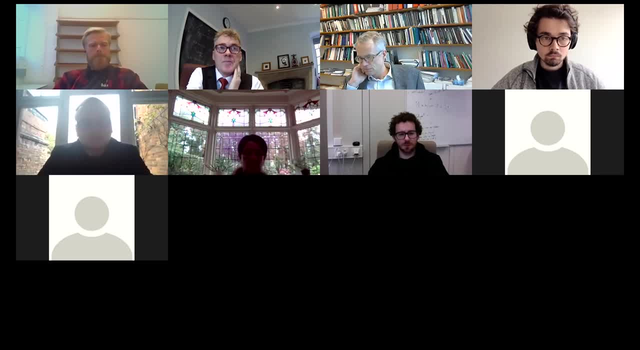 Uh, background that you're building it in. Yeah, And that's just the model of CFC minus without power set, And it's a way of maybe understanding what's going on in your remarks, at the end of your talk, I think. 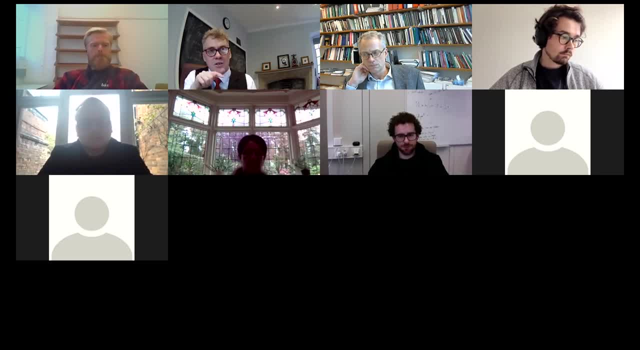 So so the, the, the countable models of CFC, countable transitive models of CFC are getting bigger, bigger, bigger, bigger. but in the limit you don't have CFC anymore. You have to give up power set because you can always be adding new subsets of. 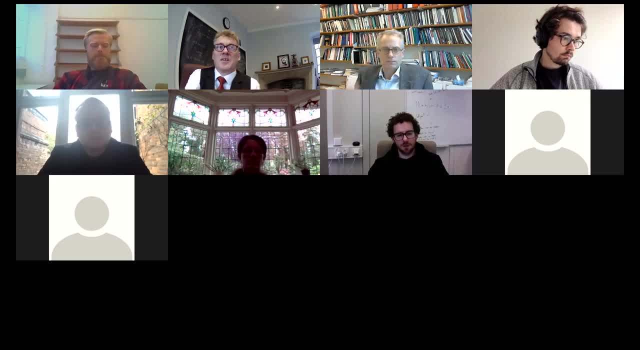 to omega, as you pointed out, And so, in the end, the power set of omega doesn't do anything. It doesn't exist in the limit model, but it still exists as a structure and it is there And it is the limit in the 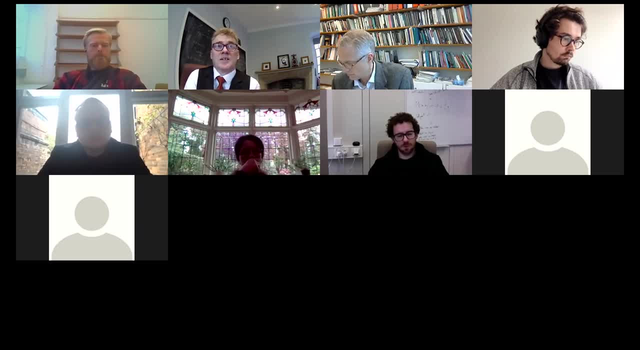 in the formal sense of the potential is limited. that I see And I defined, you know, paper, And so the the limit of those kind of transitive models of set theory is just H omega one And it's a CFC minus model. 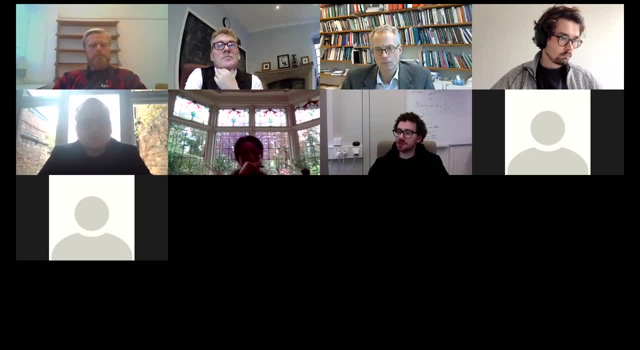 Yeah, I guess. So that's super interesting, I guess I guess my question was was- was maybe more more clearly this: is there a natural way to combine with potentialism with with the modal collapse principle? The claim is: the modal collapse principle fails. 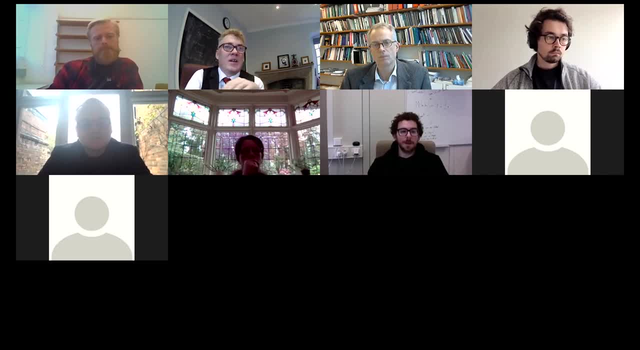 It does have modal collapse, because any subset- I mean- okay, You're talking about polar quantifiers and so on- with any subset of it exists in a larger one. So that that's going to give you modal collapse. I think So. 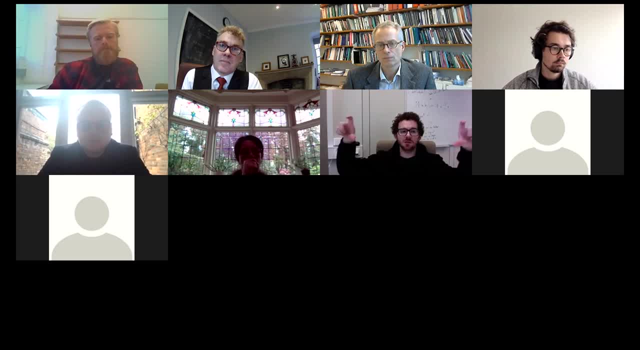 so the thought was: look look at the generic where you take these two things to, to look at the partial order over which you have your two generics. It will be an actual subset of that, Not from the perspective of the model, I know. 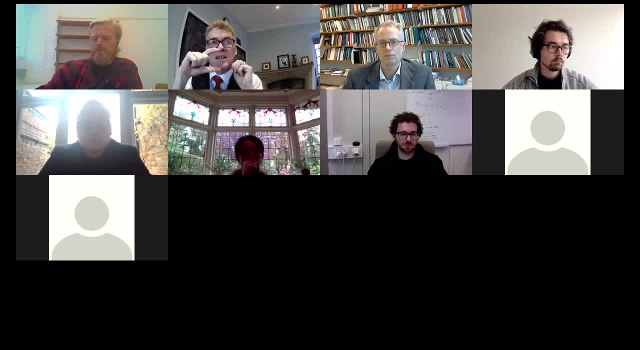 but then amalgamation is, is, it's, it's it's not saying that they can't ever be amalgamated, saying that they can't be amalgamated in a model of the same height. That's right, That's true. 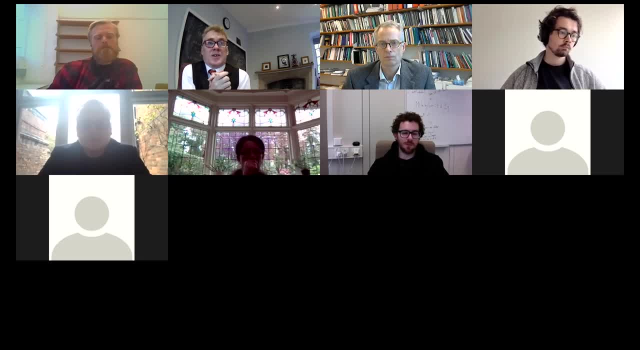 Yes, And so the way this potential system that I was just describing isn't restricted in that way And it can get taller. Oh, I see, Okay, Okay, I think about that, Thanks. Thanks, John. Uh, maybe I could ask. 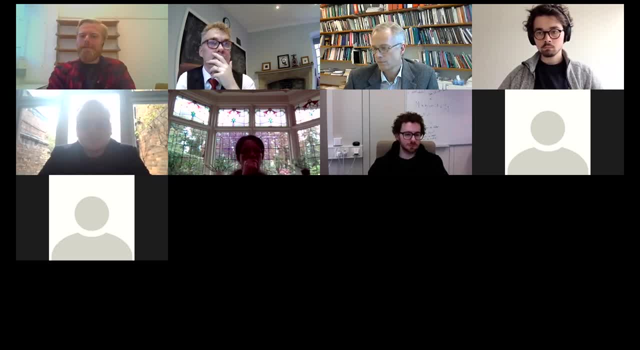 uh, I also had a question. I don't see anything in the comments, So I I just had a question about this, So maybe it comes from the me not understanding. So, or this Monty, when you started the. 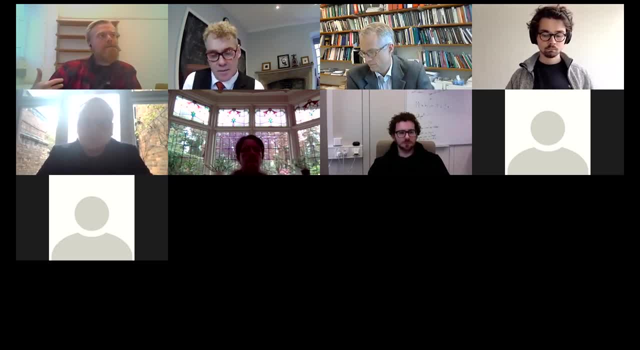 the potential system defined by Monty, because then it seemed you said: it's you, it's nice to have convergence, It's nice to have these, nice at your very properties, While in the context of these separate potential systems you've talked about. 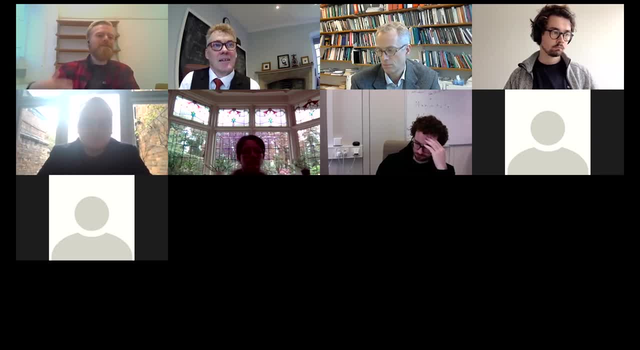 well, we maybe. you know there's a lot of, there's a lot of critical branching or or interesting systems like that. So can you talk a bit about the difference between? Yeah, I wasn't. I wasn't meaning to express a value judgment. 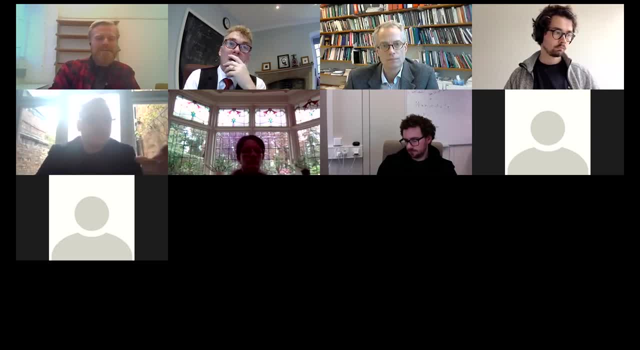 It's just that, um, I myself was confused about this for a long time. Uh, for example, the difference between directedness, convergence and amalgamation. It's very subtle, because when you have direct extension, you can't express amalgamation, even because it's the identity map. 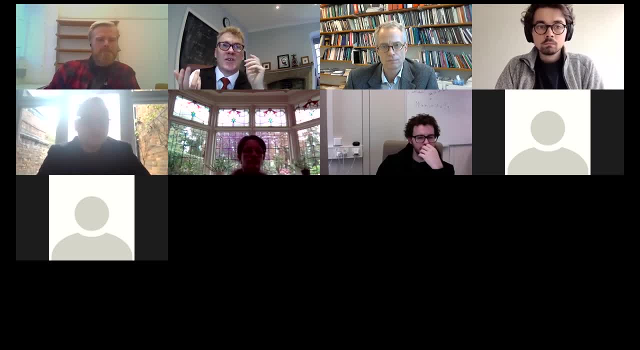 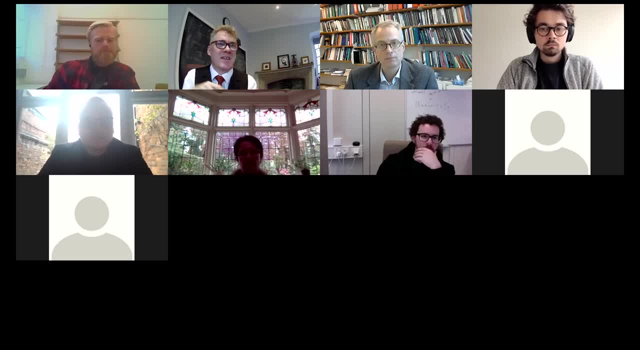 So, of course, if it's converging, then the diagram is commuting because it's the same individual each way. But amalgamation is exactly related. the commutativity of that diagram is exactly what you need in order to accommodate parameters into S4.2 validity. 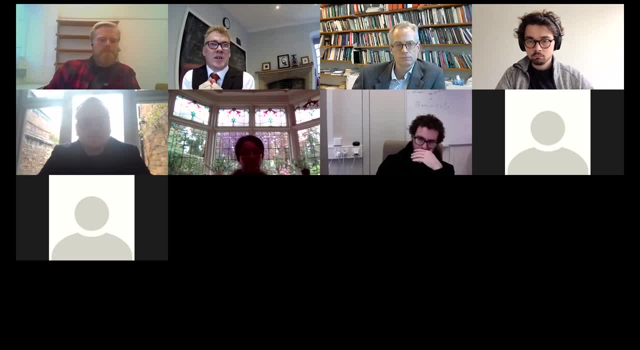 And so really you only get the S4.2 validity with parameters when you're thinking about embeddings, And it's the embedding ones that have the nicer algebraic closure amalgamation property, like graphs, for example. If you extend a graph this way and extend a graph that way, then you can put them together. 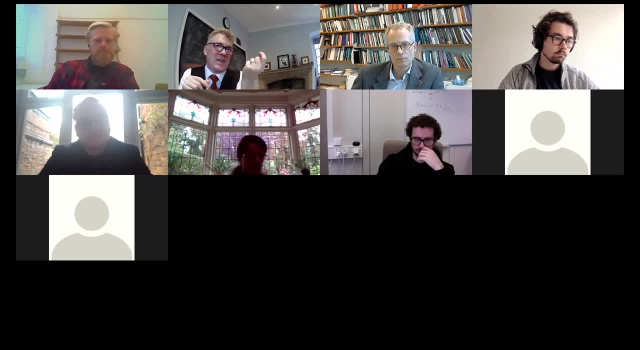 But not if you want direct extension, because maybe the actual point here was Julius Caesar and then you also used Julius Caesar over here in a different way. that is incompatible and you can't put them together right. And so it's just exactly this Julius Caesar problem right of Frege. that's the obvious. 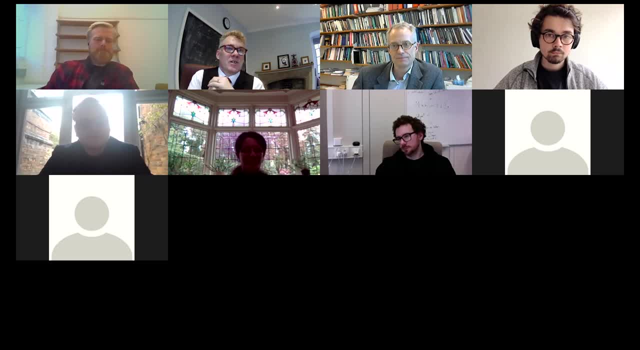 obstacle of the direct extension being convergent. And so I think mathematicians habitually don't think about direct extension but always habitually think about embedded extension, Because up to isomorphism I can put them together if I extend a graph this way and 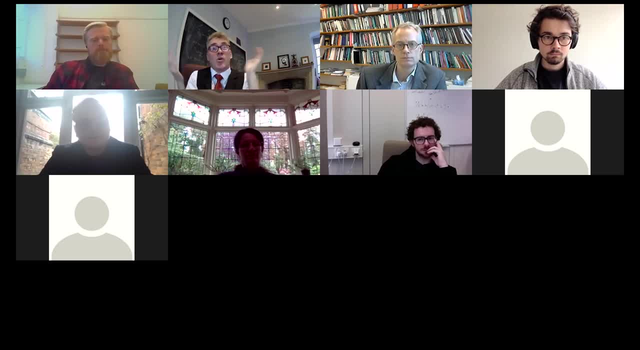 that way then I can put them into a big graph isomorphically, and that's exactly to talk about the embedding extension, And so I think one in order to get straight on the roles of what's valid with parameters and without. 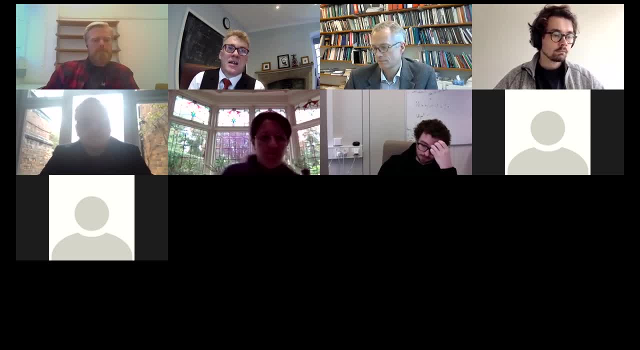 You have to really make this clear distinction between direct extension and embedding extension. I wasn't intending to suggest that somehow. I always like S4.2, and that's a superior algebraic closure. I mean when, in the context of mathematical systems that we think of as having amalgamation. 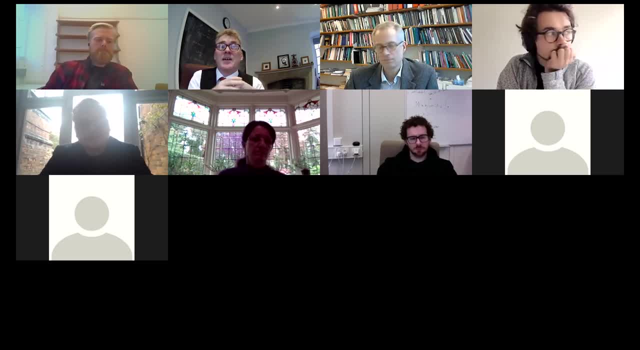 like graphs, and they do only with respect to an embedding extension- then we look upon that as a superior algebraic property And fortunately then it shows you that the embedding modality gives you S4.2, but because embedding modality is the same thing as direct extension modality, because of the theorem